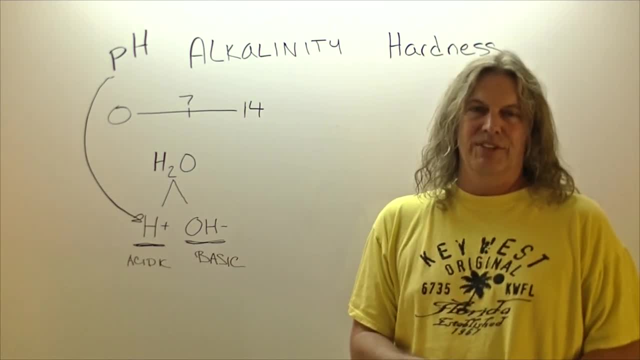 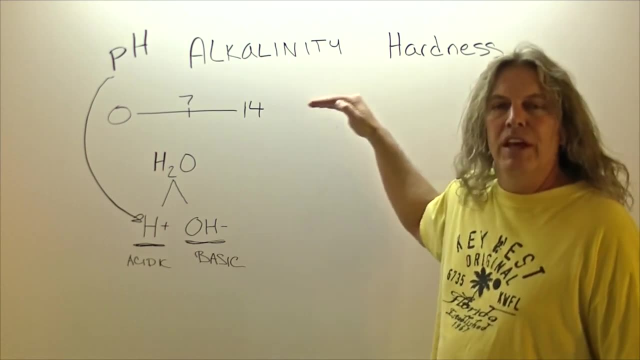 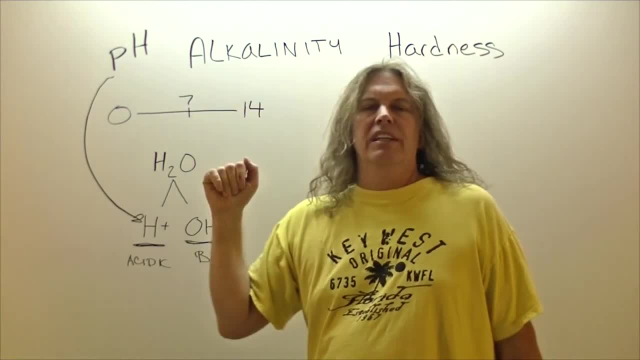 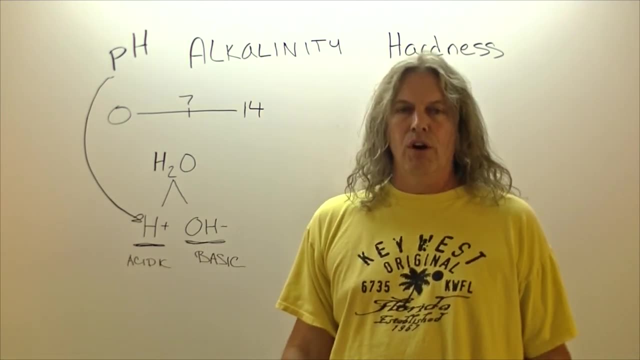 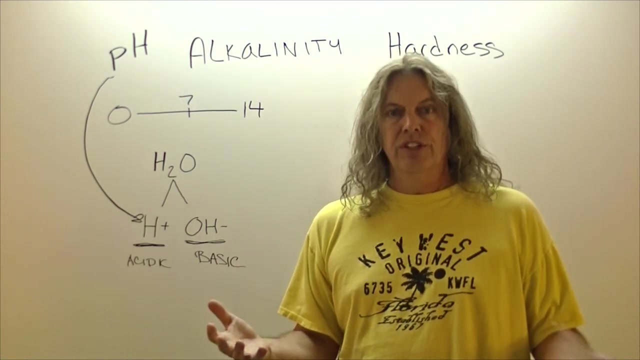 do it. Why should we care about this stuff? Well, pH and alkalinity are two basic tests that you can perform to test for the health of water, and they affect many things, including water hardness and including corrosivity. Abrupt changes can also be signs of water quality issues, such as 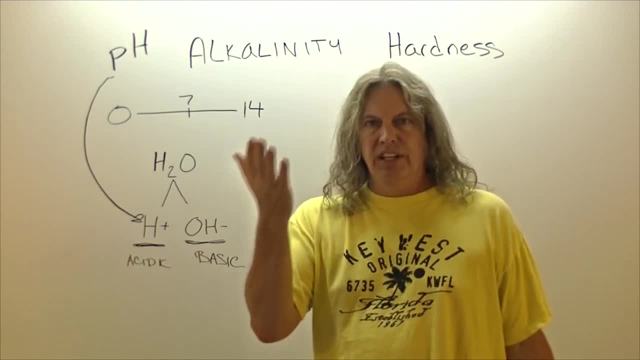 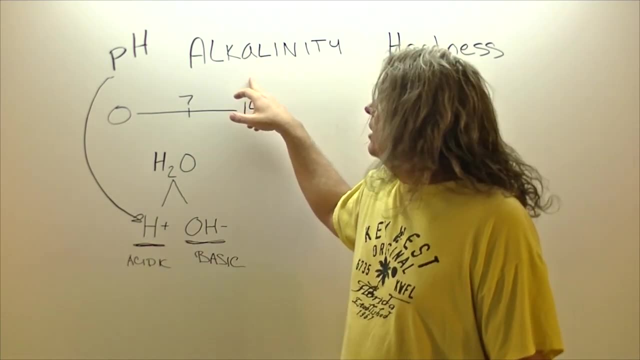 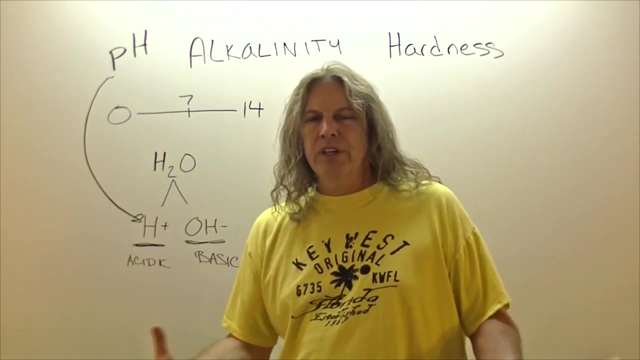 nitrification. Now, in nitrification, basically what you have is a nitrite and a nitrate-oxidizing bacteria that consume the alkalinity in that water. In the process of consuming that alkalinity, they create acids, and acids can drop the pH noticeably. So, just for an example, if you have a 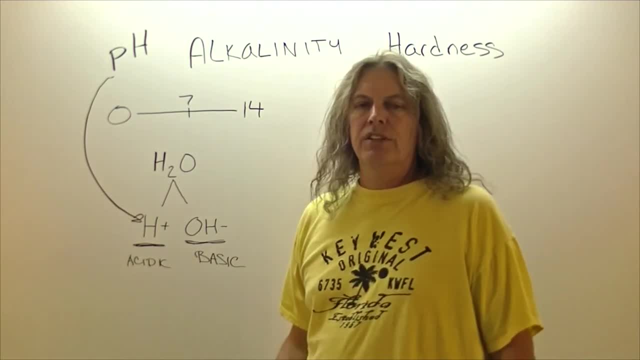 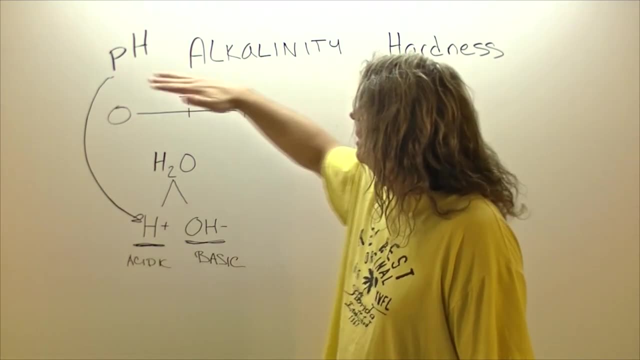 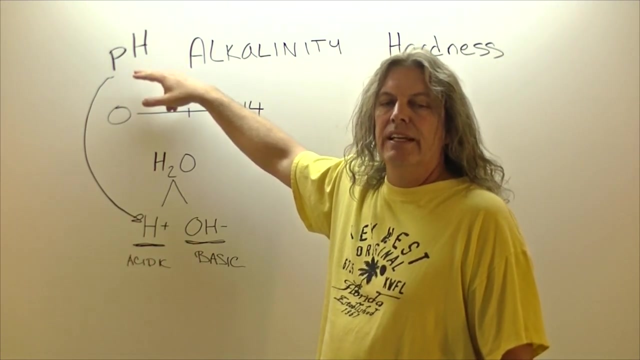 sudden drop in alkalinity, a sudden drop in pH, it can be signs that you have nitrification going on in your system. We're going to start by defining pH and then we're going to jump to the definition of alkalinity. What pH is, is it's a measure of an acidic or basic nature of a liquid, A measure. 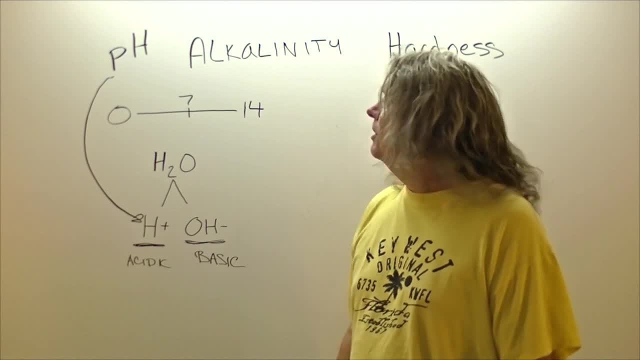 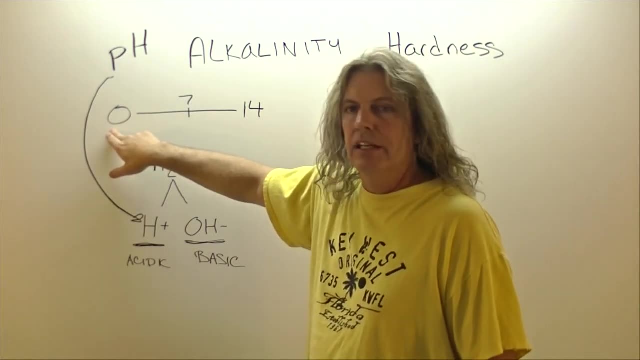 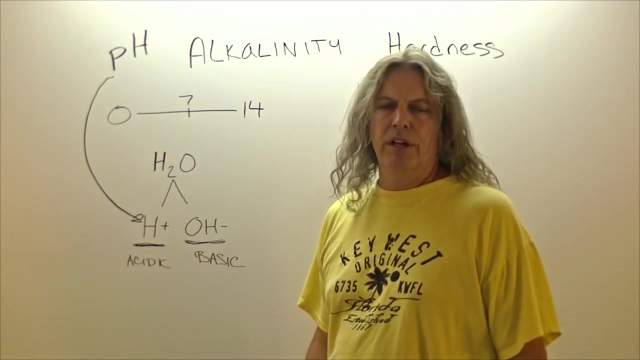 of the acidic or basic nature of a liquid, and it's quantified on a scale that goes from zero to 14, with zero being most acidic, 14 being most basic and seven being neutral. right in the middle, right there, A low pH water is undesirable, because having that acid in the water can cause corrosion. 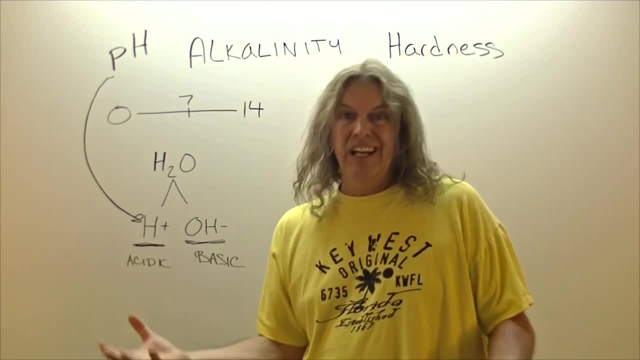 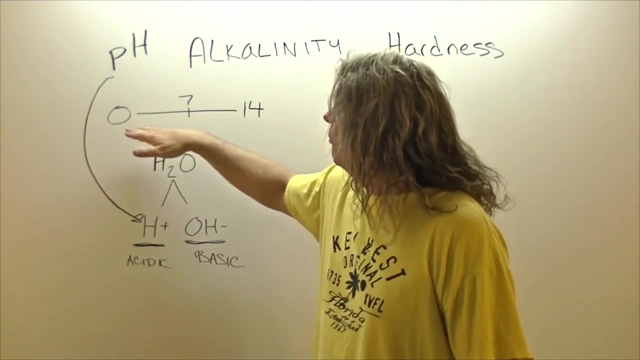 in the mains. It can cause well, the corrosion in the mains can cause holes in the mains. It can cause damage. It can cause damage to the water. It can cause damage to the water. It can cause a lot of money and repairs and damage from holes and main leaks and things like that. But over and 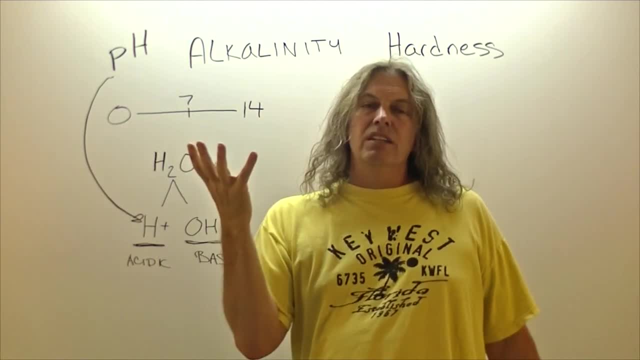 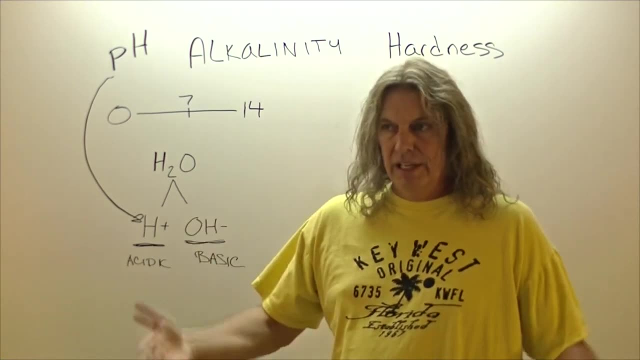 above that, an acidic water can cause a leaching of harmful things like lead and copper out of pipes and that can leach that into the system and into the water and they get into us and they're bad. So there's a lot of reasons we don't want acidic water- Water that's too basic. on the other hand, 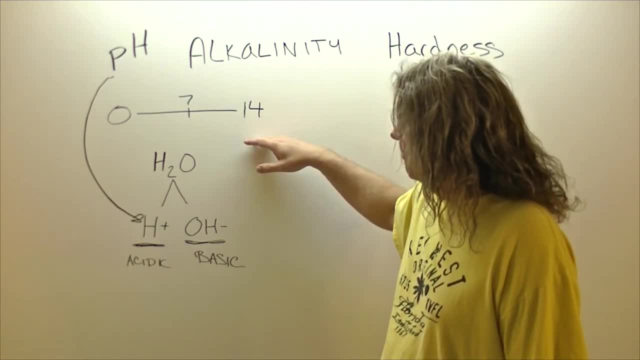 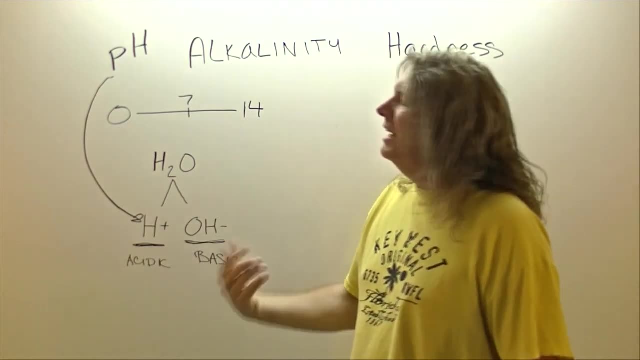 has other things that can go wrong with it, like deposition of scale and so forth. Now I want to take it another step farther and talk about how acidic water can cause a lot of damage to the system. I want to talk about this symbol right here. Okay, we get it. It's a measure of an acidic 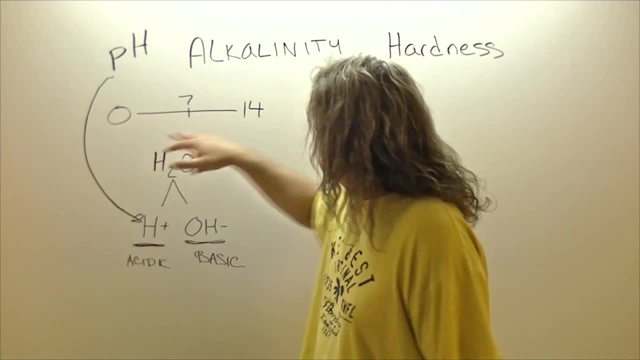 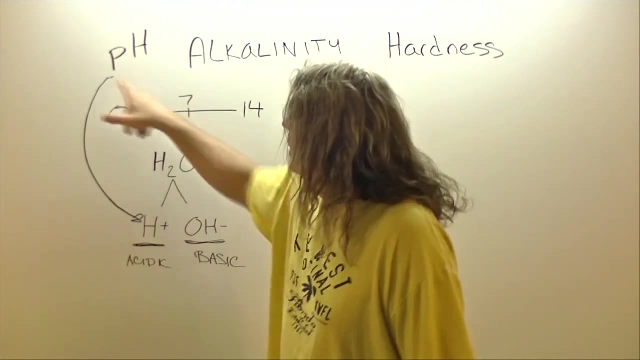 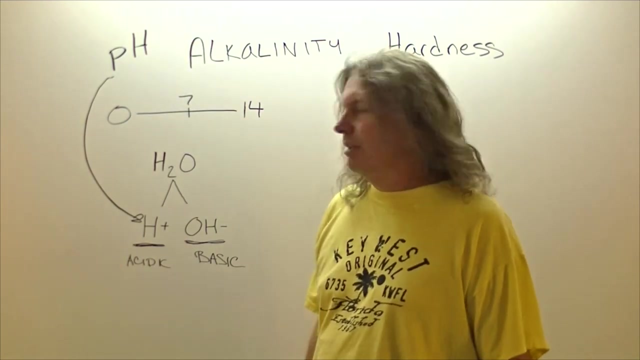 or basic nature of water. Zero is acid, Fourteen is basic. What does that mean? What does that mean what I just said? Well, pH, and the reason why it's written kind of funny like that is because it actually stands for the power of hydrogen, the element hydrogen. Let's take that and break that. 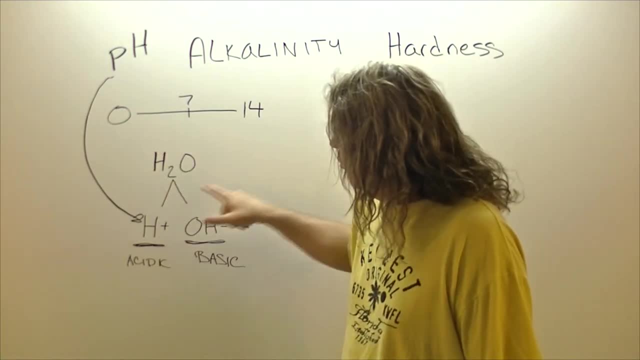 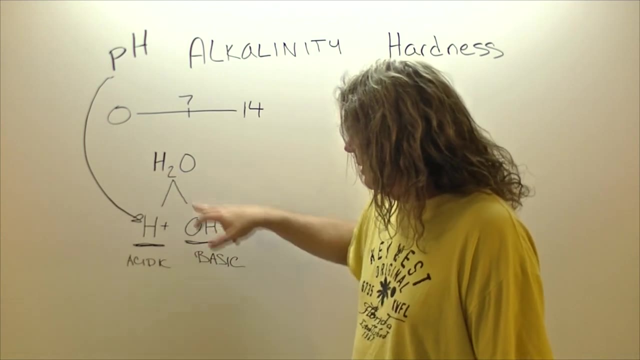 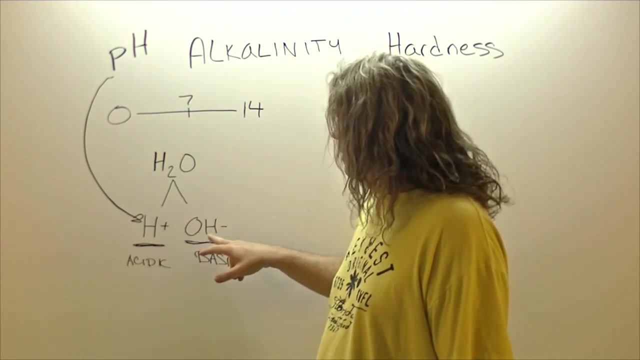 down a second and then we'll come back to that. So we have water right here, H2O, and certain amounts of that water can break apart into the hydrogen ion And it can also break apart into the hydroxide ion. The hydrogen ion is acidic, The hydroxide ion is basic. So pH, the power of 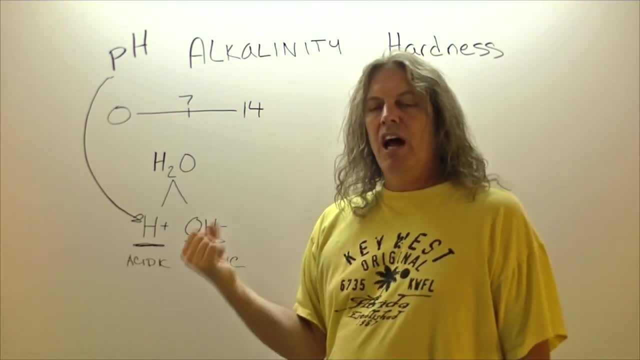 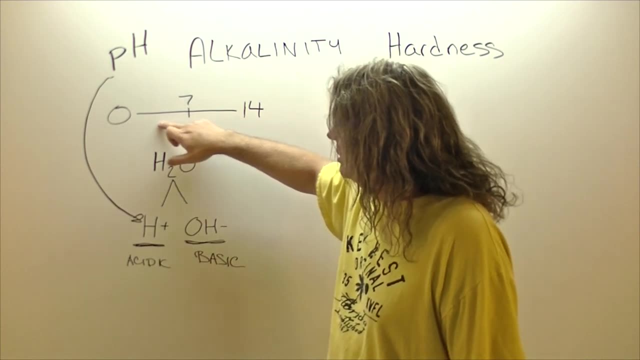 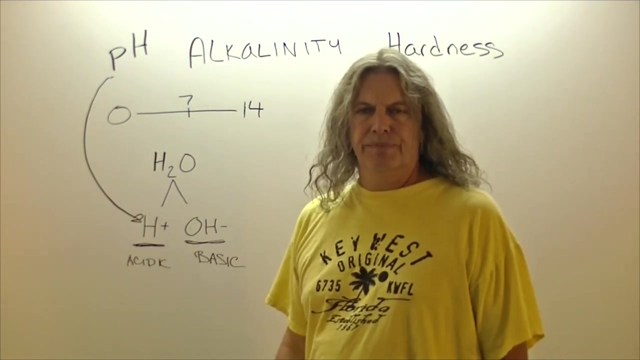 hydrogen basically measures the amount of hydrogen ions that are floating around in that water. So the more hydrogen ions, the more acidic a solution is. The less hydrogen ions ions, the more basic a solution is. Let's talk about these acids and bases for a. 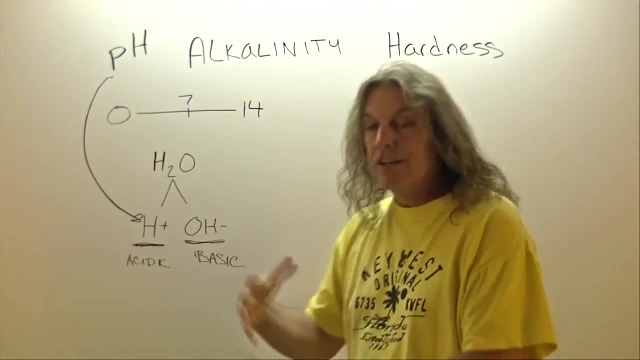 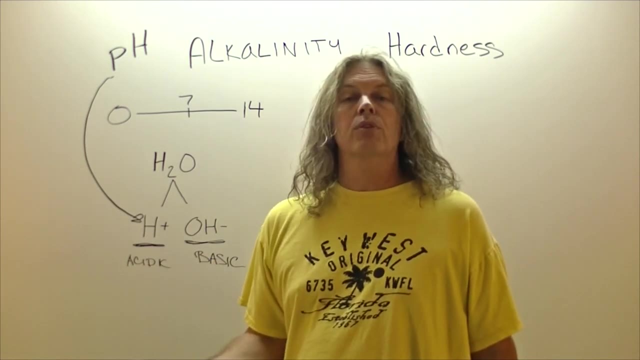 second, just to kind of recap that a little bit and add to it a little bit: Acids are solutions that supply hydrogen atoms. I'll give you an example: Hydrochloric acid, HCl. it can break apart into that hydrogen ion and the 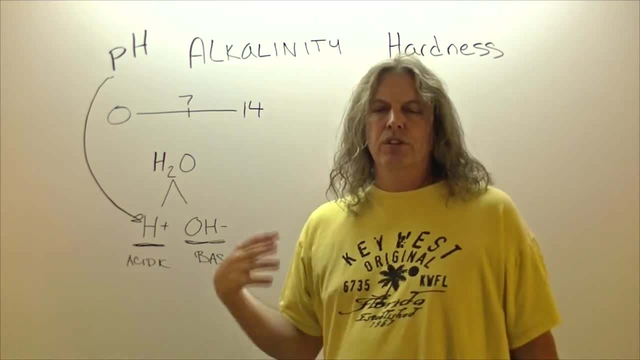 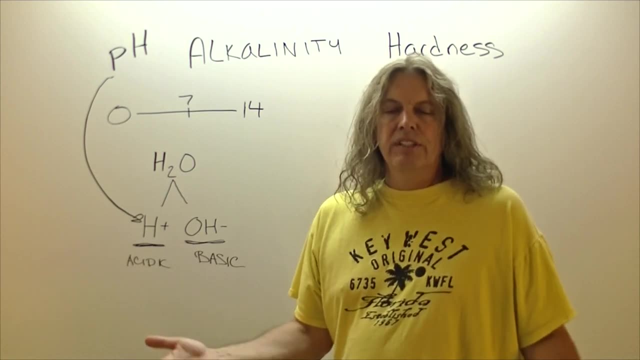 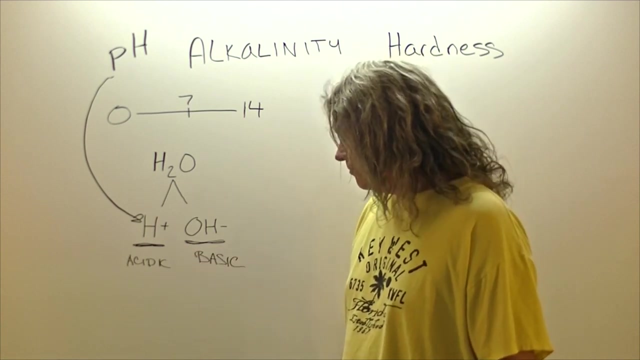 chlorine ion. Bases, on the other hand, are solutions that provide hydroxide ions. I'll give you another example of that. Sodium hydroxide can break apart into the sodium ion and the hydroxide ion. So if you ask yourself, well, what's water? Is it? 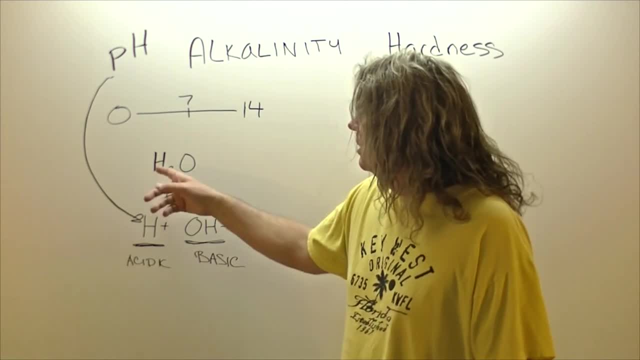 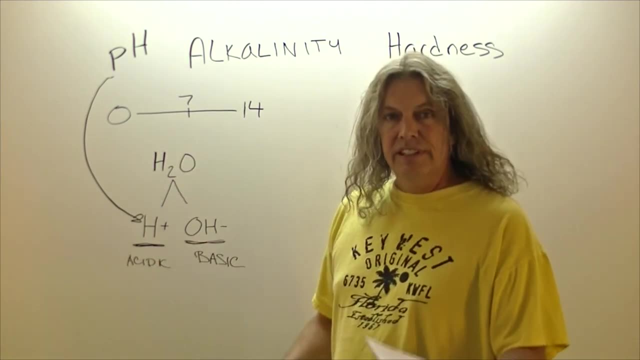 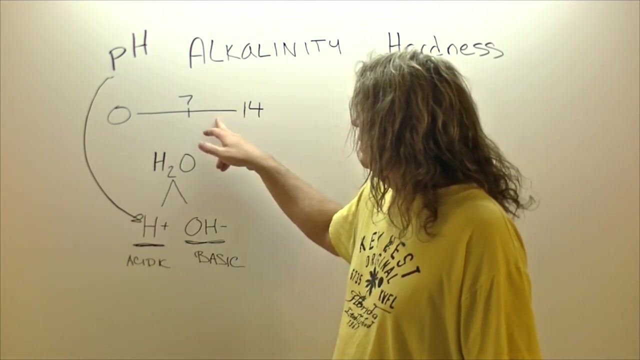 an acid or a base. Well, distilled water is neutral because the hydrogen ion is counteracted by the hydroxide ion and it's exactly neutral. So distilled water would have a pH of seven, which is neutral. Natural source waters are about six and a half to eight and a half because bases can be picked. 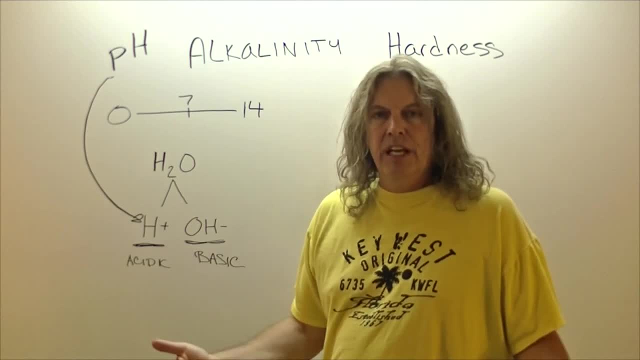 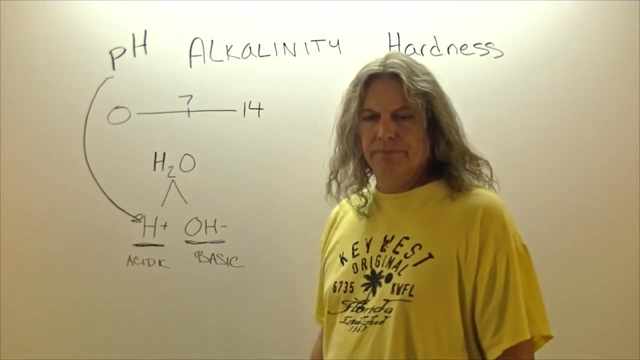 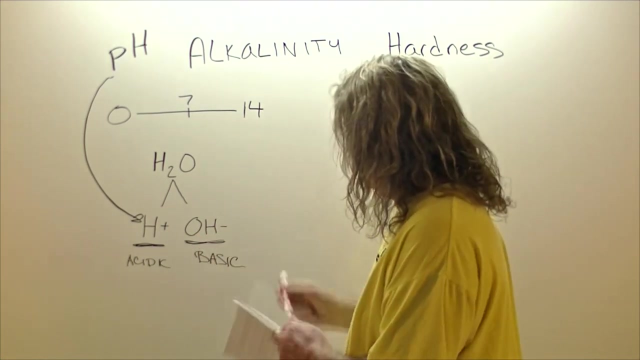 up as water runs through- you know lime, for example- as water runs through the ground and so forth. So water, natural water, tends to be just slightly basic. One thing- I want to talk about this before we move on- is this: OH, negative. 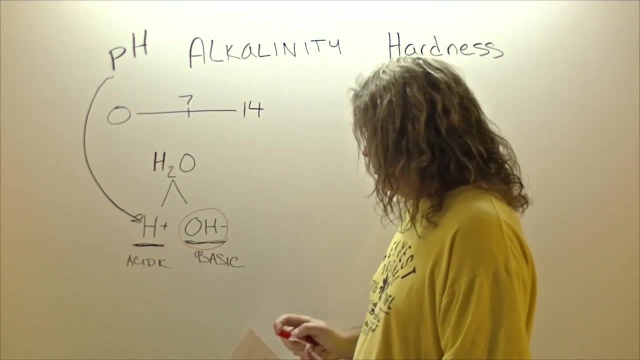 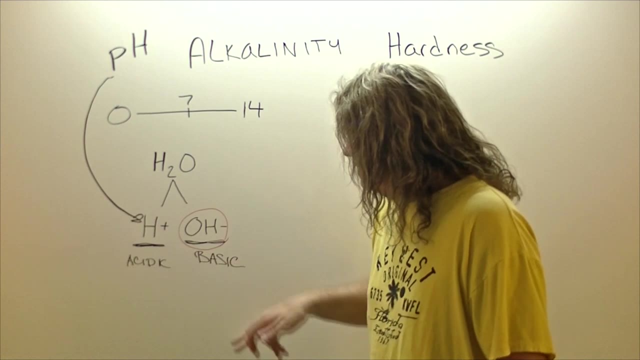 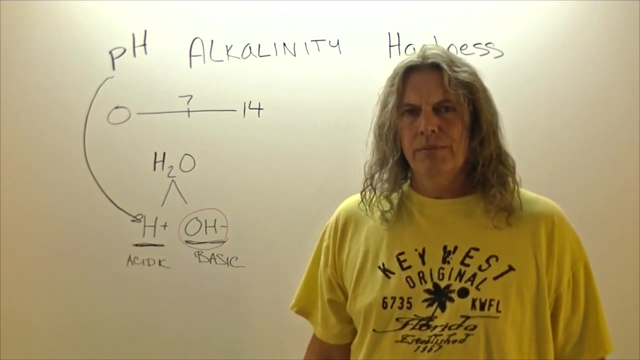 the hydroxide And when I was first learning this. I just want to clarify- this is kind of like a side note thing that we're going to come back after that- But the hydroxide, I saw the OH negative and one time I was actually teaching a class over at San Jose Water and somebody said: 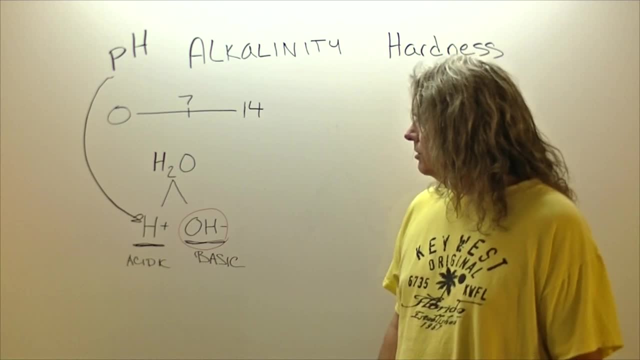 isn't that a hydroxyl? I said: no, it's hydroxide, He said: but it's a hydroxyl, it's OH negative. So I didn't know what the heck he was talking about. This was way back in the day, So that's. 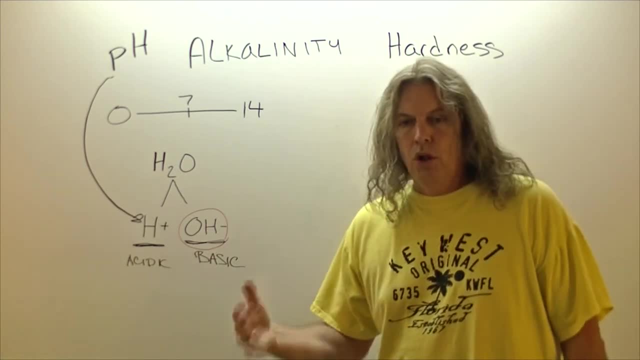 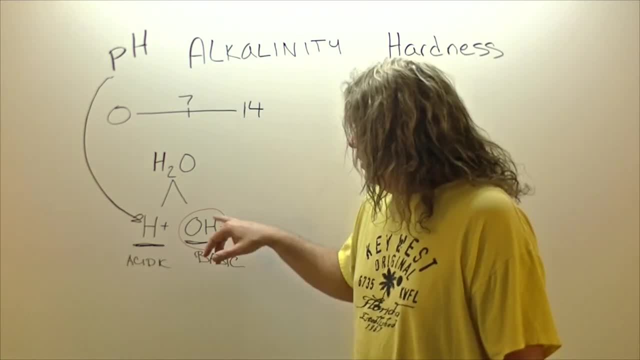 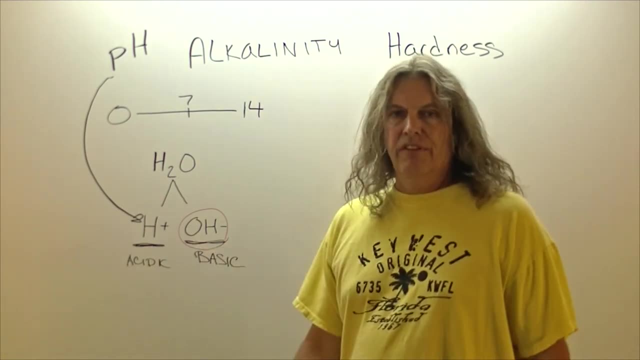 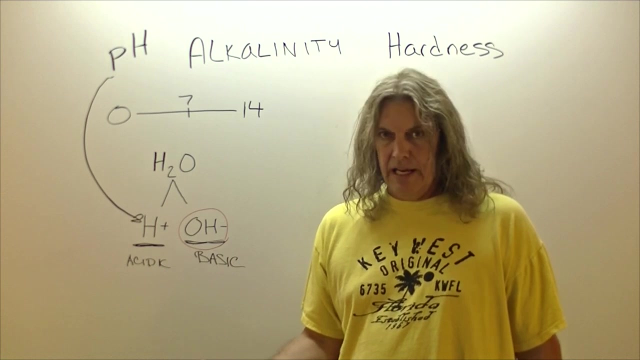 hydroxyl, spelled with a YL at the n, is basically the exact same thing: OH negative. the hydroxide is the exact same thing, OH negative, And you'll see this written all over the place, sometimes as hydroxyl and sometimes as hydro présent, and people mistakenly call it a. 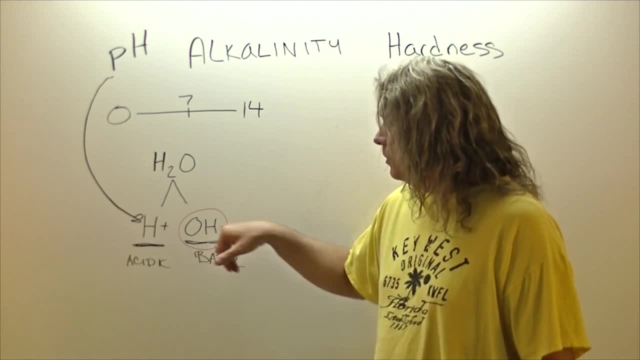 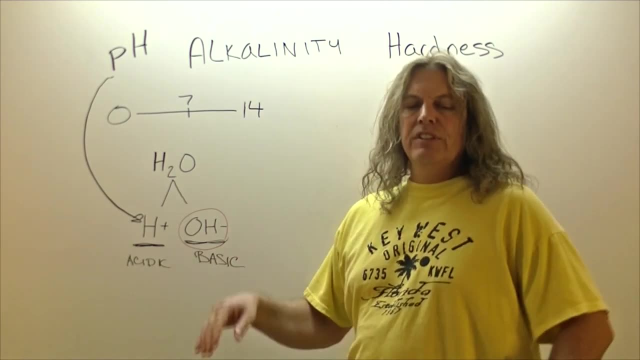 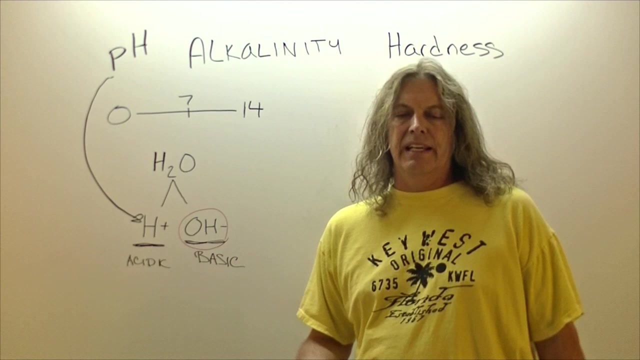 hydroxyl when they're referring the bases right here. The proper term for that is the hydroxide in a book. I just want you to understand. They look exactly the same. The difference is the hydroxyl is generally when you use this compound in terms of organic chemistry. 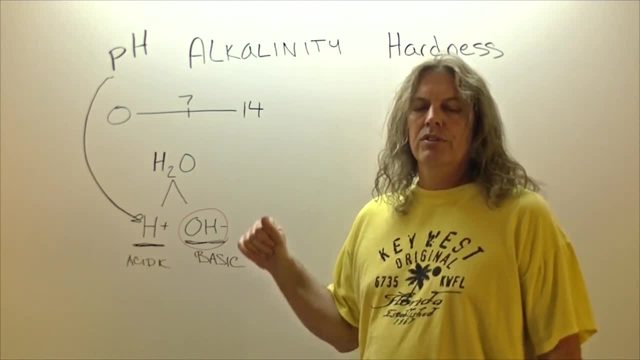 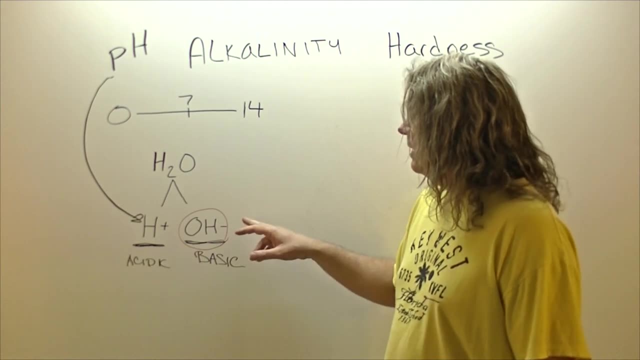 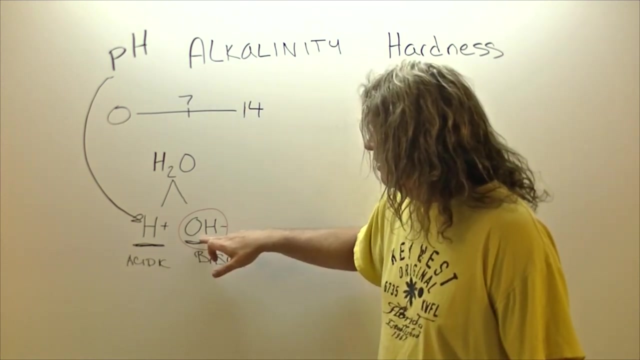 containing the element carbon, and most hydroxyls pertain to things like sugars, alcohols, and they are not basic meaning. when you take a hydroxyl compound and dissolve that into water, it will not break up to provide an OH group Hydroxides. on the other hand, what we're dealing 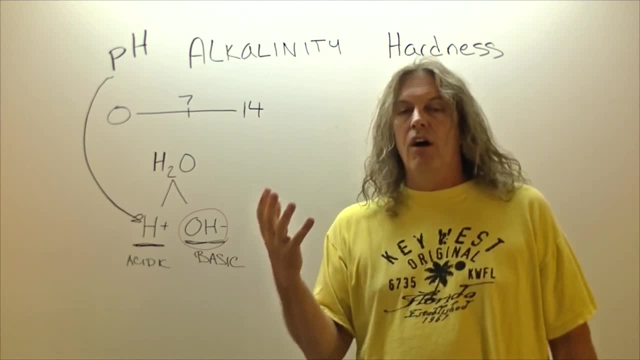 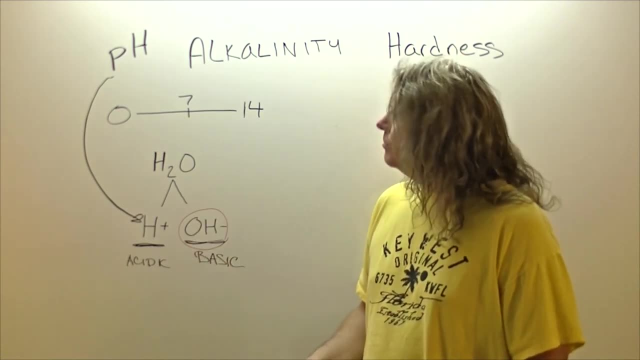 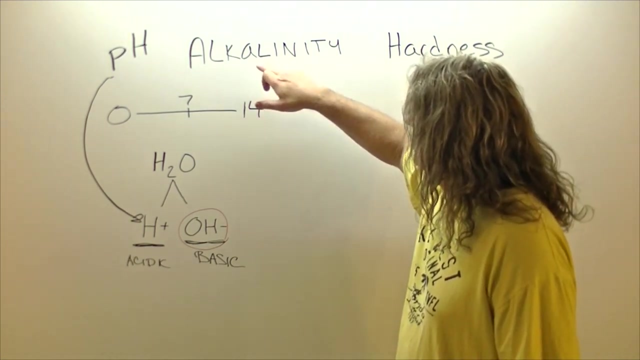 with is actually a term for the inorganic compounds that are classified as basics, meaning they do break up and provide an OH group when dissolved in water. Let's take a step forward now and let's move on and talk about alkalinity, And when talking about alkalinity, I want 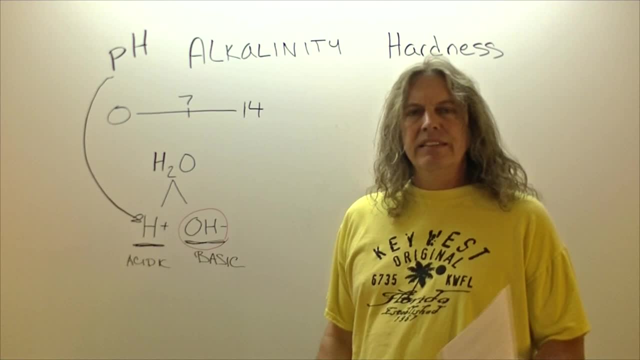 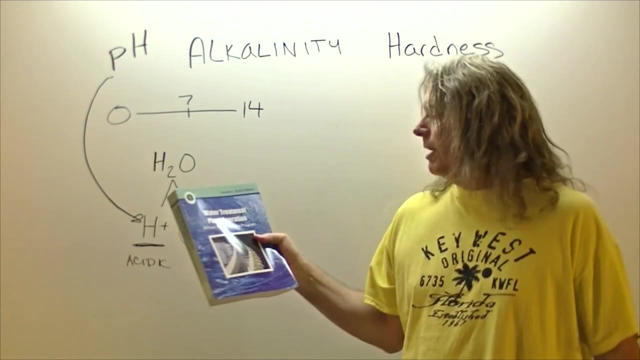 to start by just defining what alkalinity is. When I talk about alkalinity, I want to start by defining alkalinity. There's a fantastic book that I talk about and I rave about this book all the time. I'm not trying to promote it here- I don't get that into promoting- but 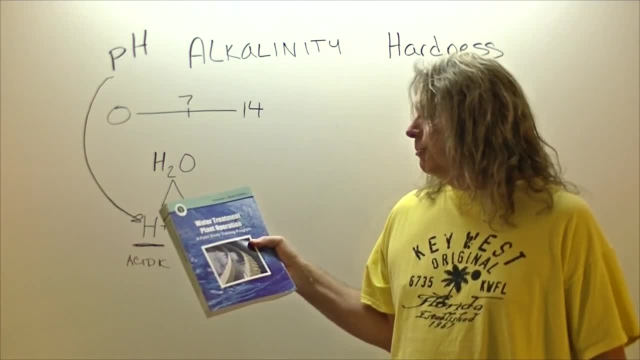 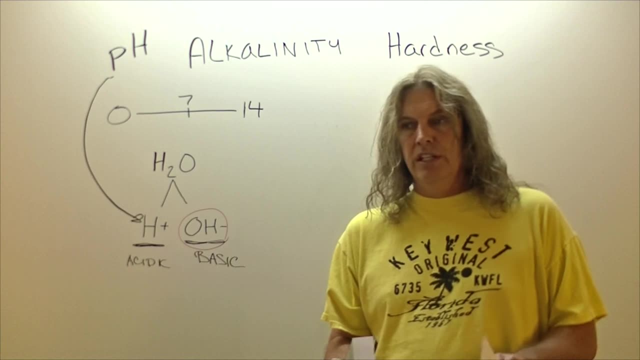 Sacramento State University has a home study course you can take: Water Treatment Plant Operation, Volume 1.. It's a course I recommend people take, by the way, as a prerequisite if your state requires a prerequisite to taking your treatment exam. It's also a fantastic. 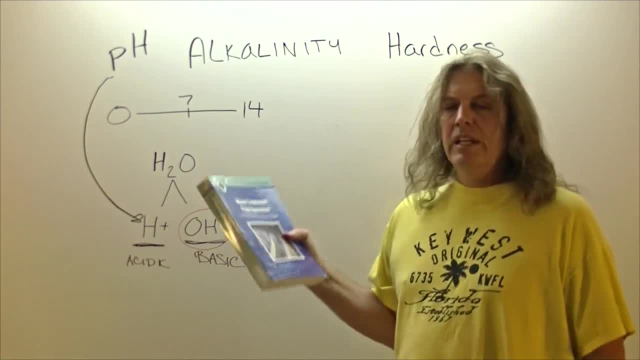 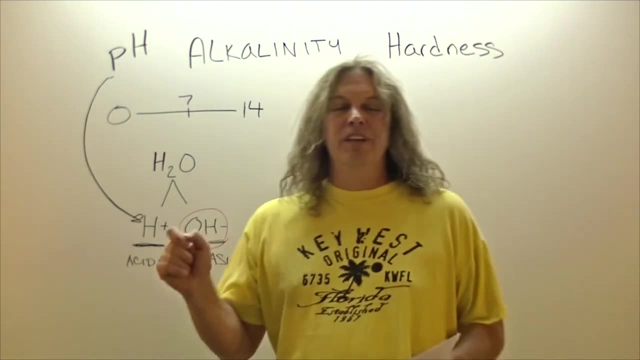 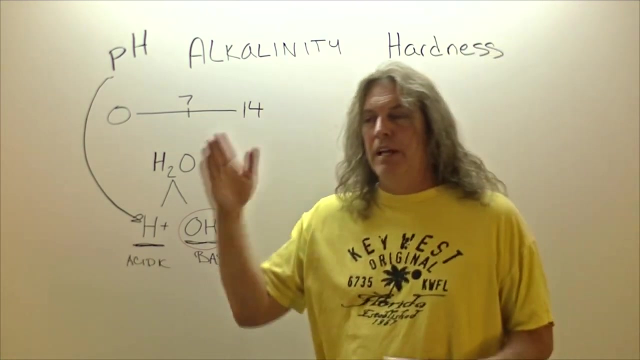 course to take for continuing education. Anyway, it has three definitions in that book. It has three definitions in that book when it talks about alkalinity. And we're going to go through each of those three because I feel like by going all three of them it kind of helps beat it in. 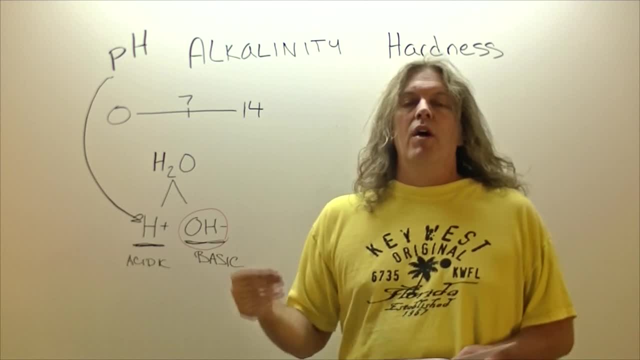 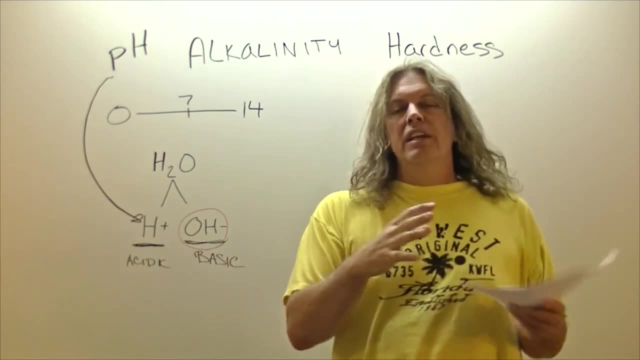 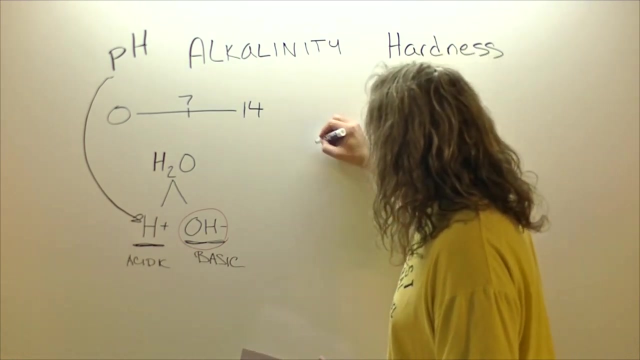 One of those definitions in alkalinity is the capacity of a water to resist a change in pH. How alkalinity does that is it reacts with any additional hydrogen ions that are floating around and neutralizing them. Okay, so if you have a floating around hydrogen, 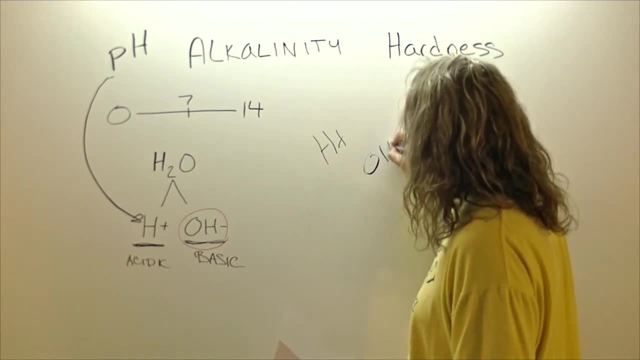 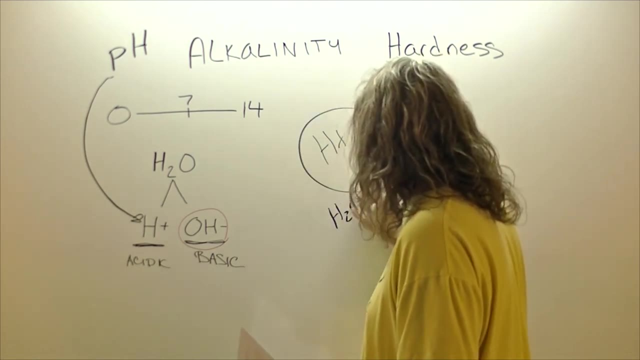 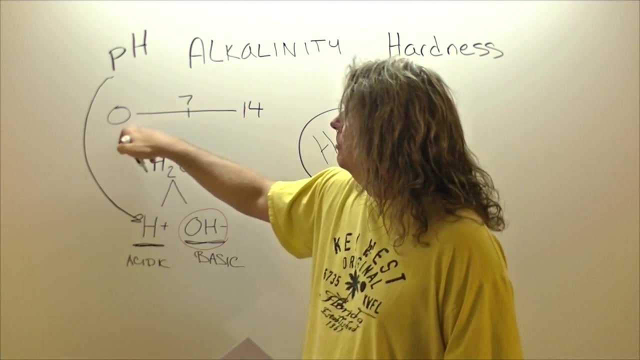 ion there and you have a floating around hydroxide there. that hydroxide and that hydrogen can combine together- Let's say it forms back into water, for this example here- And therefore that extra hydrogen ion has been neutralized. It's not floating around as an acid to make. 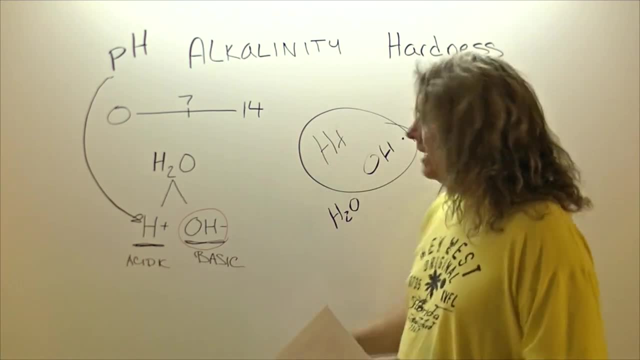 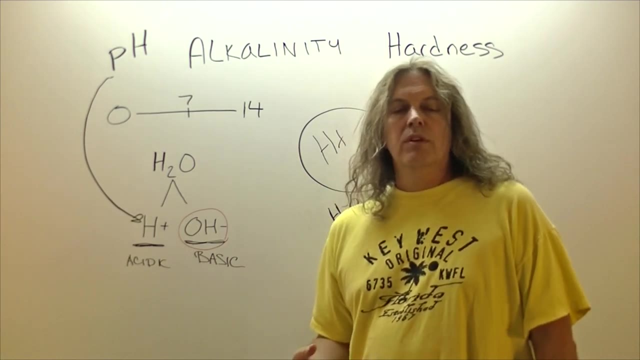 that water more acidic. So again, getting back to that definition, the comparison between alkalinity and alkalinity is a very obvious one. It's a very obvious one. So it's a very Capacity of a water to resist a change in pH Definition to the capacity of a water to neutralize acids or its acid neutralizing. 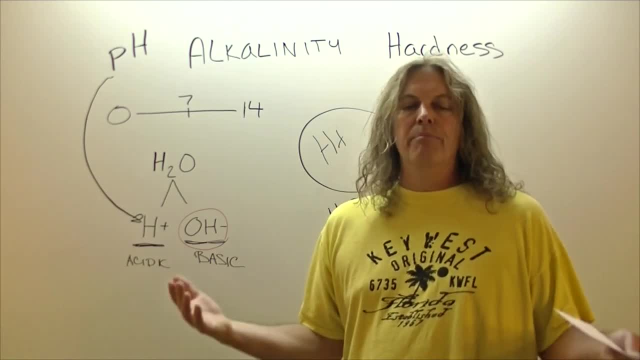 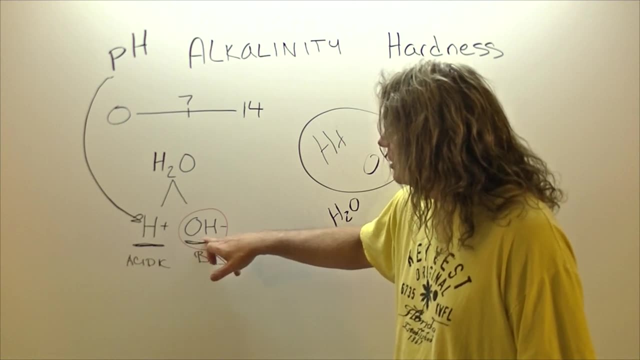 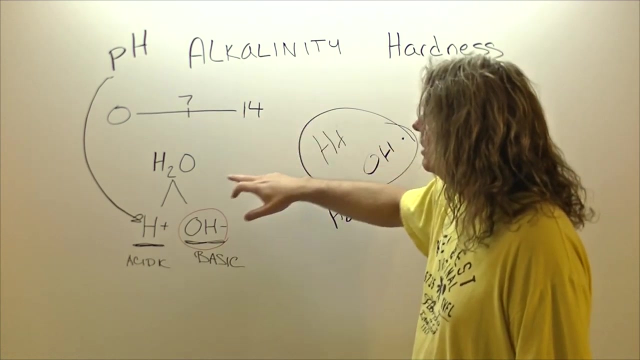 Capability, and by this it basically just means a total amount of bases that are contained in that water. The more bases you have in the water, the more things that can break apart to supply this hydroxide ion, the more hydroxides can be Free in the water to tie up with those floating around hydrogen ions. 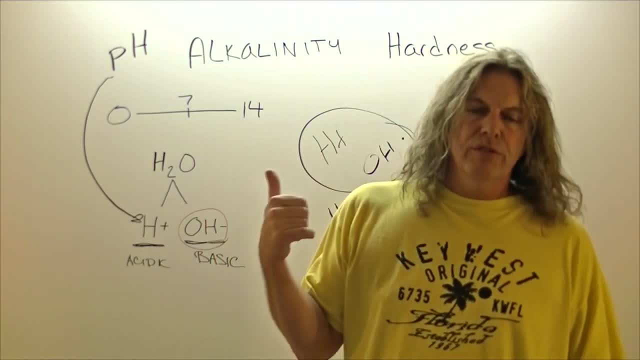 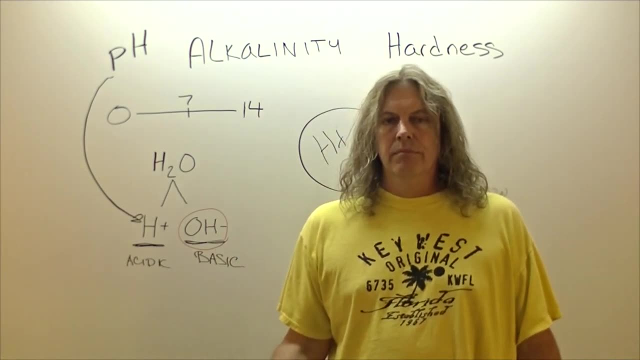 And then the third definition is a measure of how much acid must be added to lower the pH to 4.5. For the longest time I had this definition memorized. Here's the kind of stuff I'm trying to stop you guys from going through with this video for the longest time. 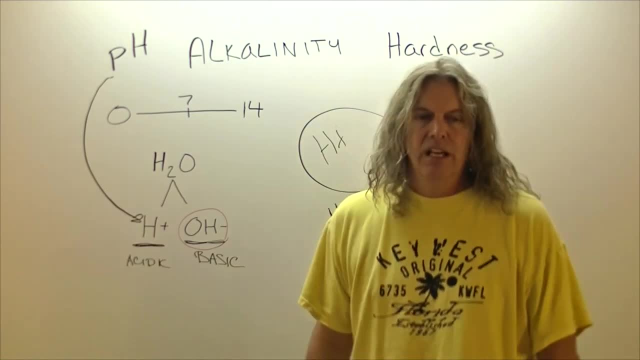 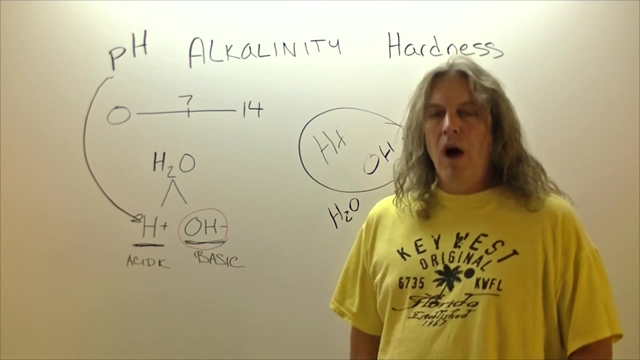 I had this definition memorized and I took tests and I passed tests. The measure of how much acid must be added to a water to drop a pH to 4.5. I didn't know what 4.5 meant. Well, why 4.5?? 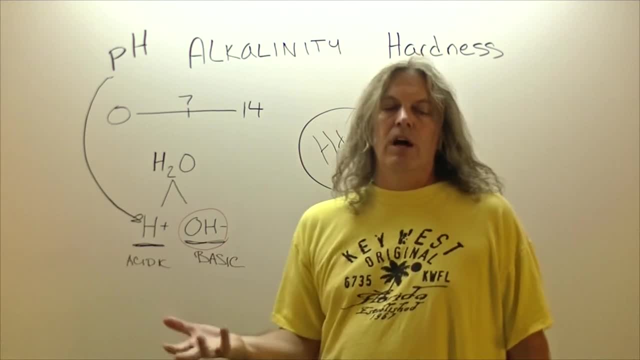 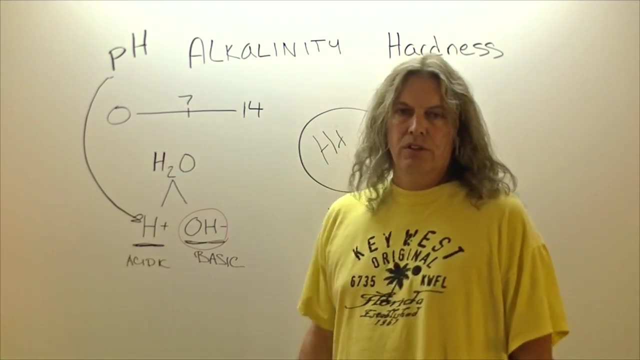 4.5 Is the point below at which you have no alkalinity, meaning all the alkalinity, all the bases that are in that water have been Consumed by the additional, by the hydrogen ions in that water. They tied up with all the hydrogen ions and now below that you have three. 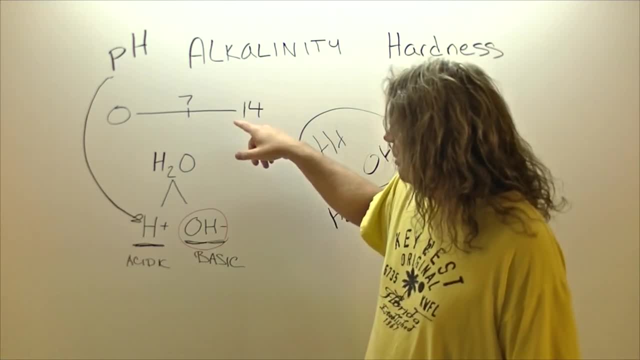 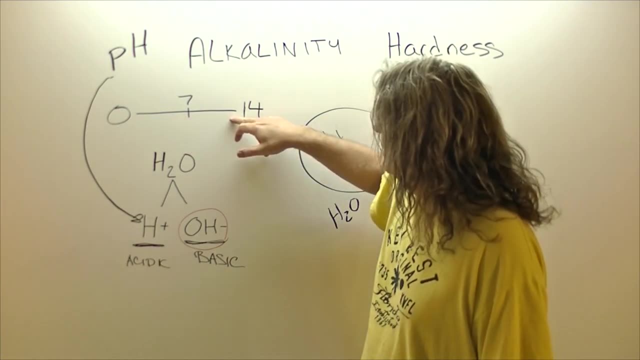 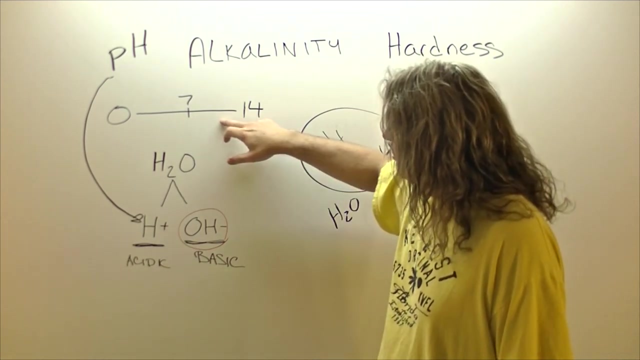 hydrogen ions. because of that, if you're ever doing a Test for alkalinity and the pH and so forth, You'll notice that as you add what acid to a water And it ties up those bases, ties up those bases, It'll drop slowly, slowly, slowly, slowly. once you hit 4.5, and all that alkalinity, all those float around. 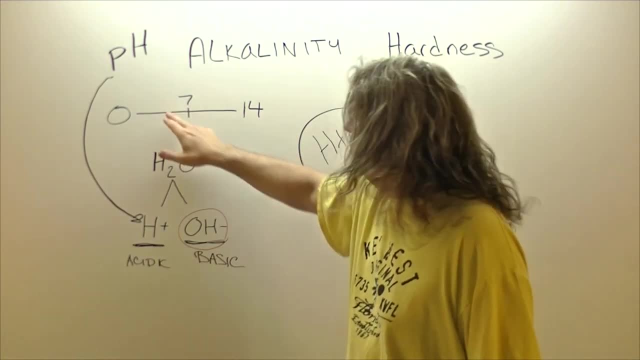 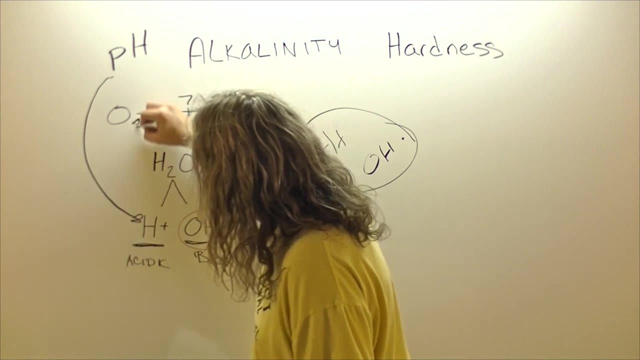 Hydroxide ions there have been consumed. once you pass that pH of 4.5, You'll notice that the pH and that water will drop really quickly, Because now you add acid to the water and there's nothing to tie it up as it's been added. if you want to see a 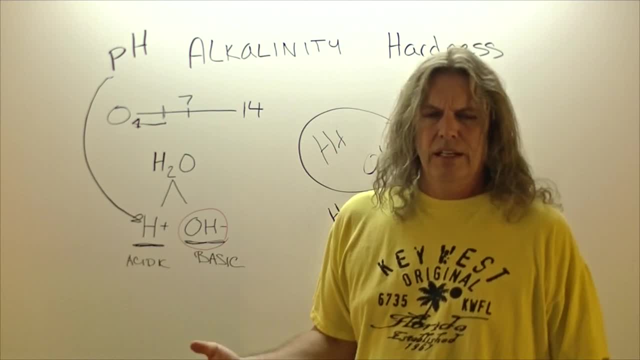 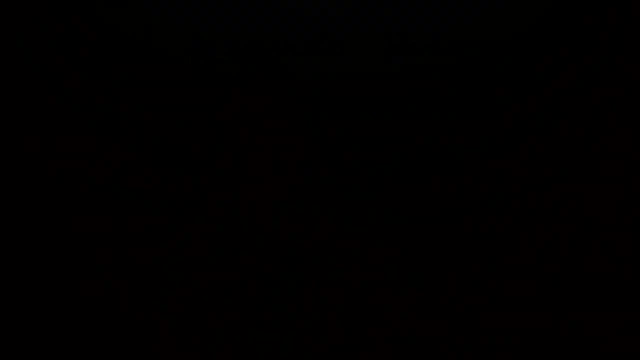 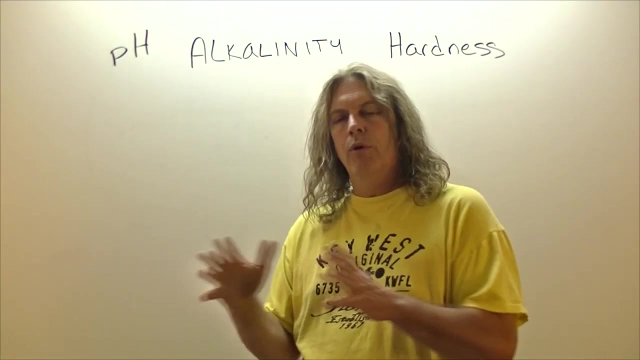 Video that go check out my video on Alkalinity. I think it's- uh, it's alkalinity test, I think is the name of the video. Let me erase this for a second. So that talks about the definition of alkalinity. Let's go ahead and talk about different forms that alkalinity can come in. 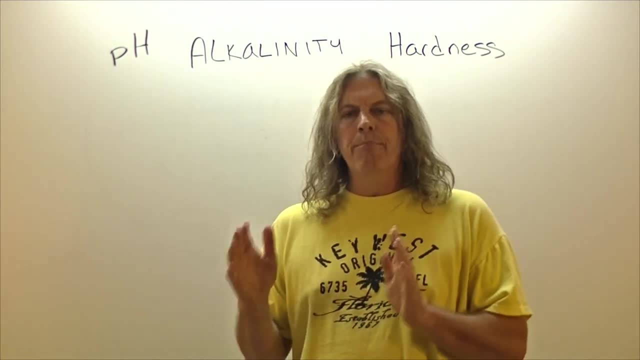 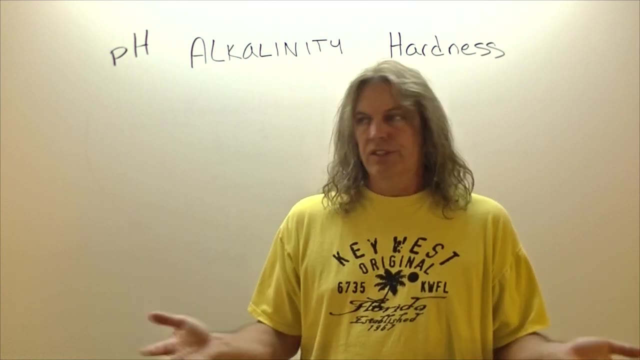 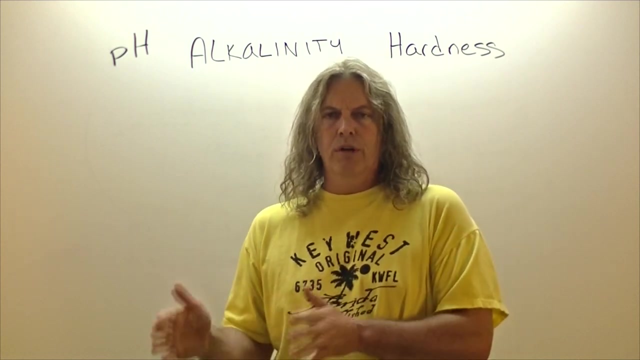 alkalinity mainly comes from the carbonates and bicarbonates of calcium and magnesium, And these are just naturally occurring minerals and metallic salts that are just kind of out there in the earth. Calcium is a naturally occurring mineral. its most common form is calcium carbonate. Which layman terms for calcium carbonate is limestone. 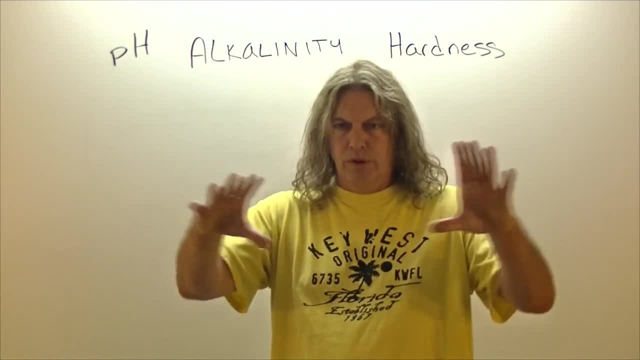 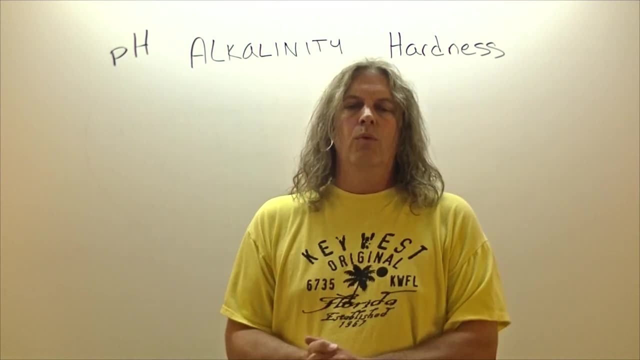 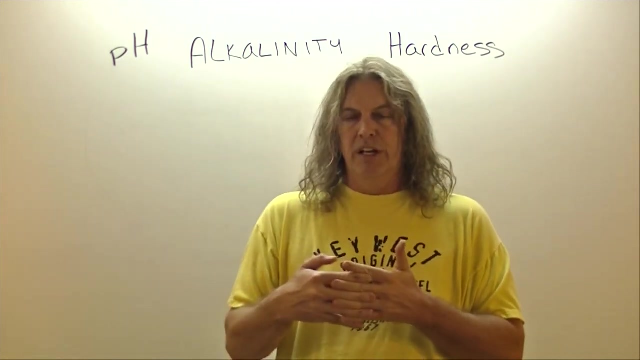 The water just kind of flows through the earth and over the earth and where there's limestone there it picks it up and that gets Dissolved in the water and combines with the water molecules and adds alkalinity to the water. We also use calcium carbonate and treatment plants. not so much specifically does it come in as calcium carbonate. 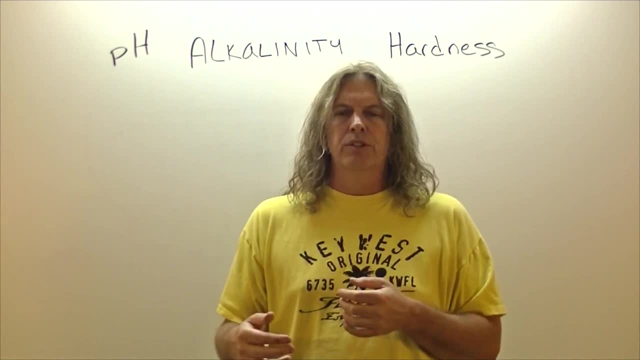 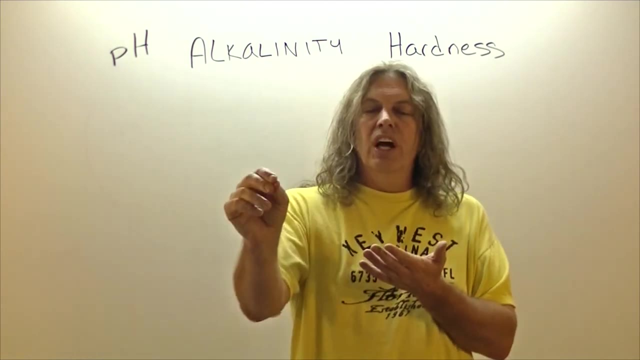 But we converted to calcium oxide because that's easier to transport and we use that as part of the lime slaking process, so that when we're at the plant and we need to Adjust the source waters, We need to adjust the pH and alkalinity. we do that. 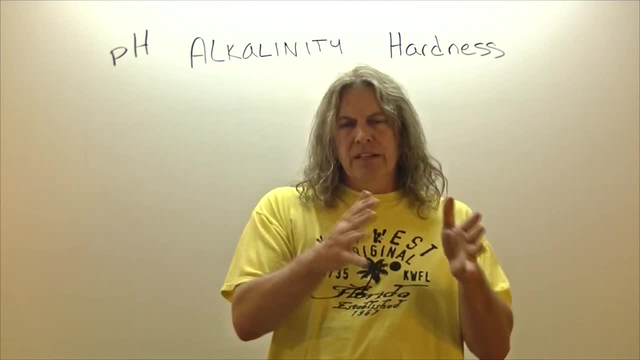 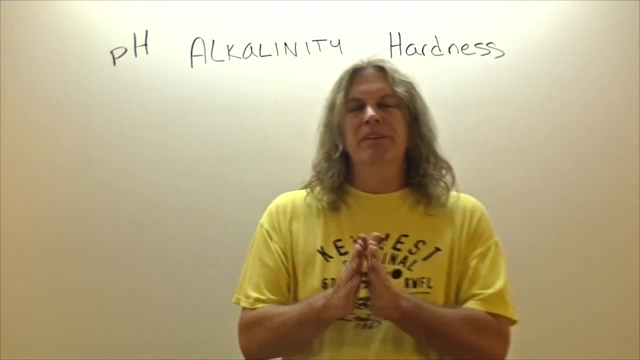 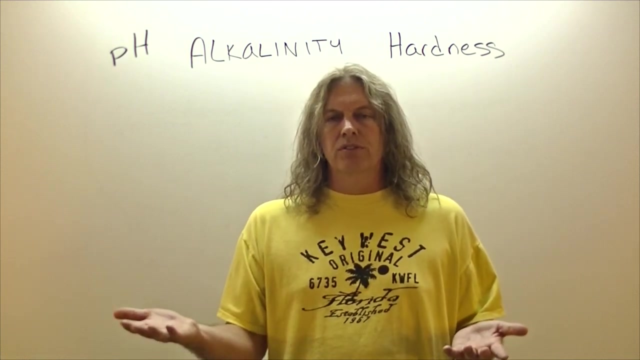 So that's, you'll see. you'll hear a lot of that from there. now getting back to magnesium again, That's just make now Magnalic been talking too much today. Magnesium is pretty much just metallic salts: magnesium bicarbonate, which is Magnus D, magnesium sulfate, which is epsom. salts are 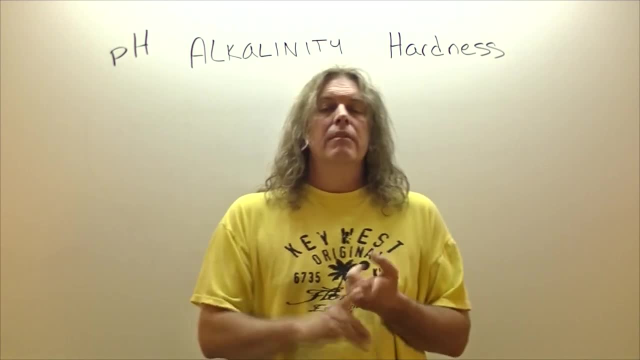 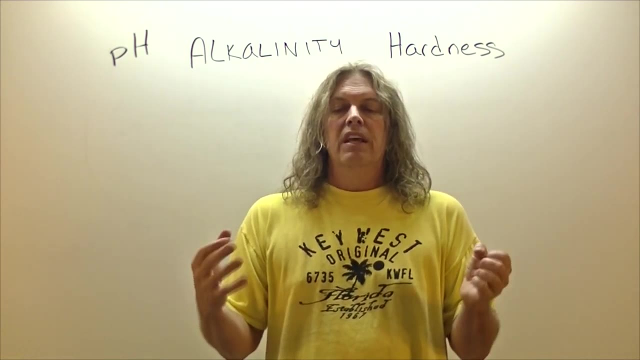 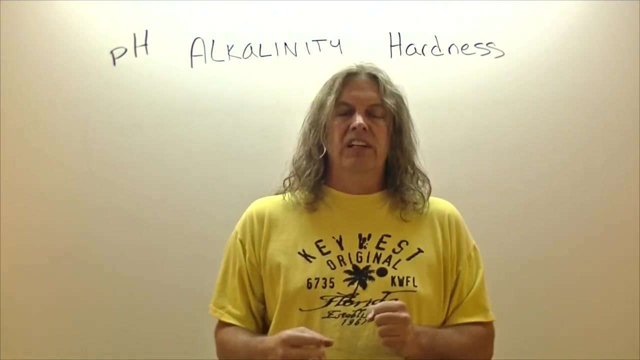 Kind of just some examples of that. so those are two things: carbonates and bicarbonates of calcium and magnesium. but there are a whole other group of things that can combine and form alkali groups or Combinations of molecules or things that have alkalinity in them, that can break apart to add alkalinity into the water. 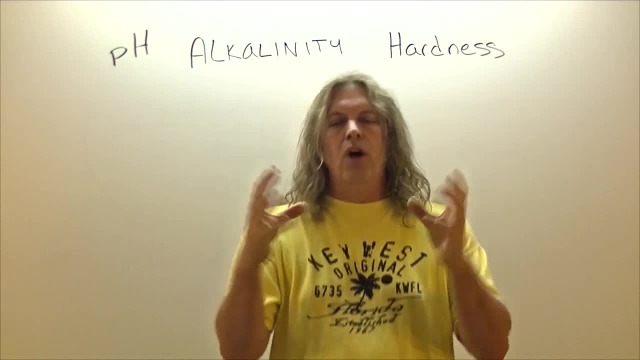 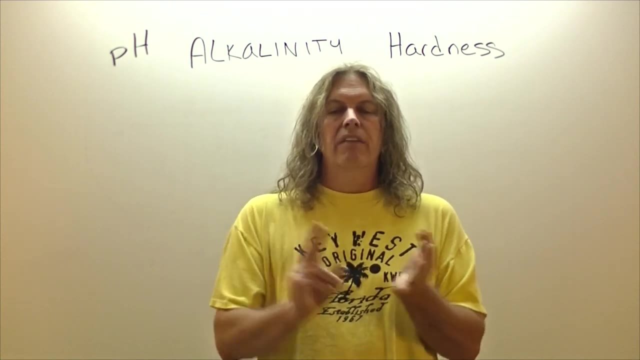 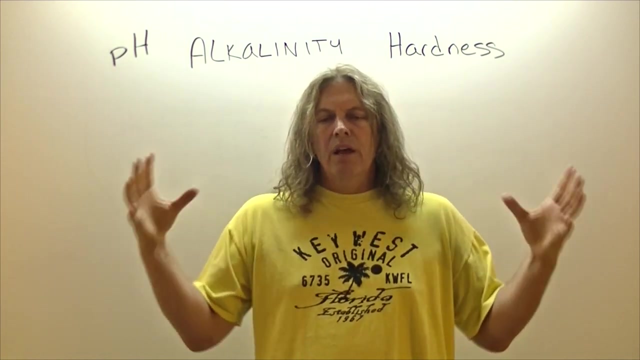 We refer to this whole group of molecules as alkalinity. some of those other things are hydroxide, borate, silicate and phosphate. so therefore, alkalinity is actually a collection of many compounds and many chemicals that can react with those hydrogen, the hydrogen ions that are raised off the board. 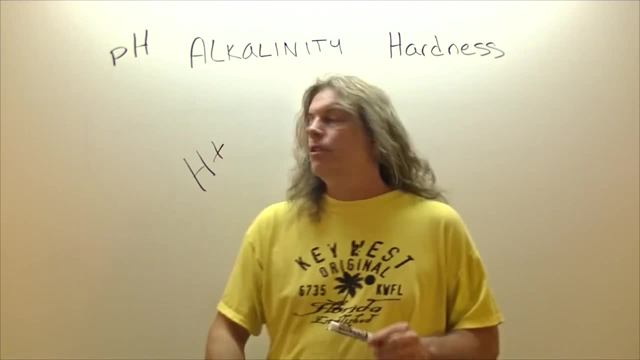 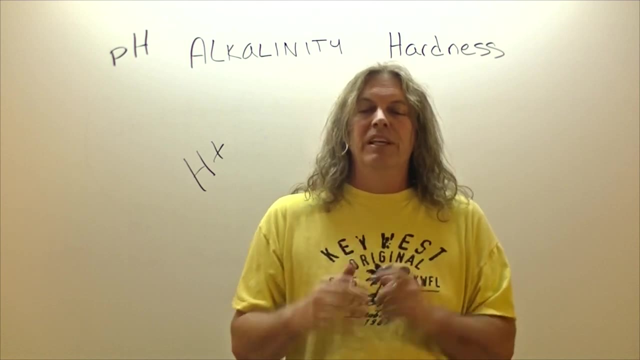 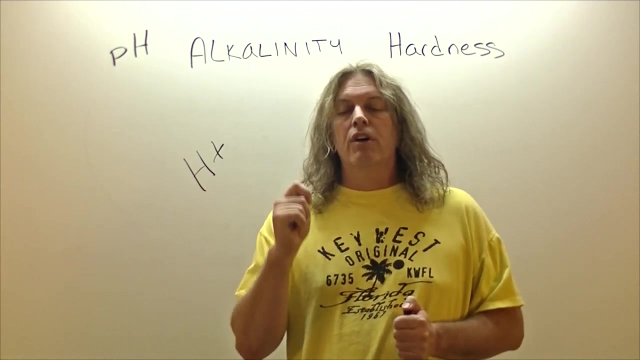 Had to put it back, So I'm not pointing nothing. They can react with those hydrogen ions and prevent them from appreciatively changing the pH of the solution. So alkalinity can take many forms, but it's measured in terms of carbonate hardness and it's expressed in 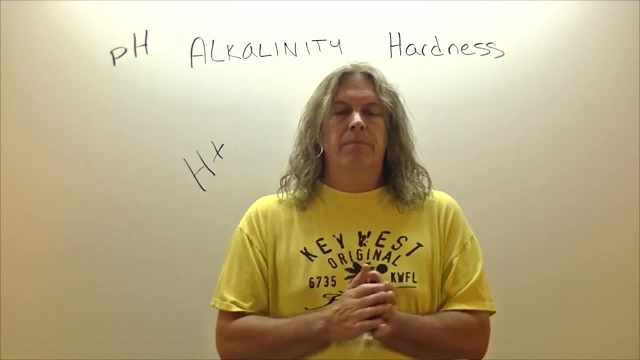 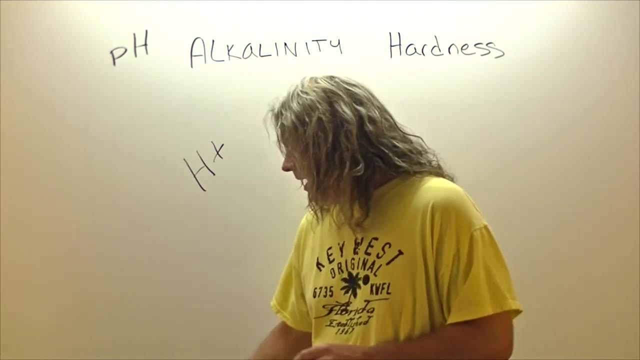 terms of equivalent calcium carbonate. Why? Because it's the most common form, but in addition to that, I like to think of it as kind of a common ground approach. If you have two meters six inches and three feet, how are you going to? 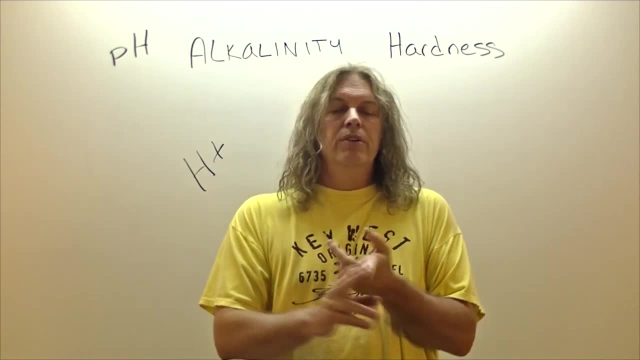 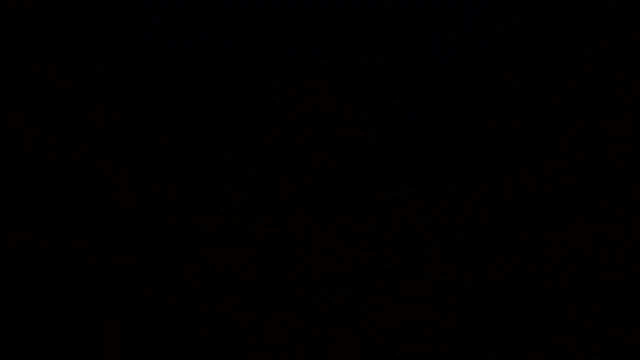 tell someone how far something is. So if we converted two meters six inches and three feet all to feet, it's a lot easier to work with. So let's go ahead and talk about alkalinity and hardness. Alkalinity, the calcium carbonate, is a. 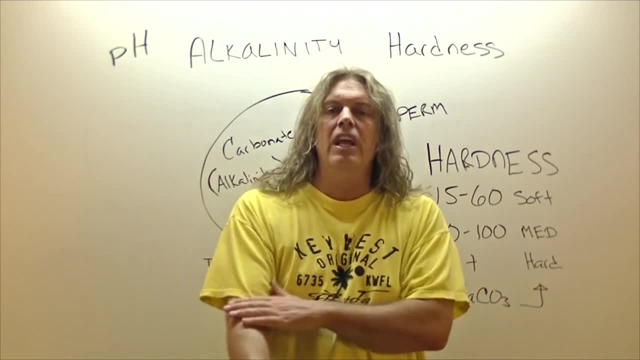 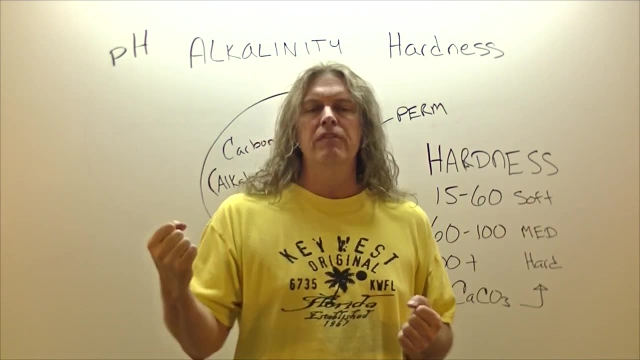 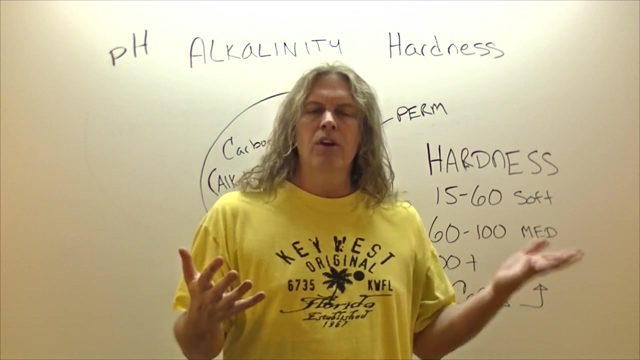 good thing It stops that water from appreciatively changing one way or another. It helps it resist that change in pH. We want to make sure we have enough calcium and magnesium to achieve that proper pH and alkalinity. However, the presence of calcium and magnesium in our water is not always a good thing. You 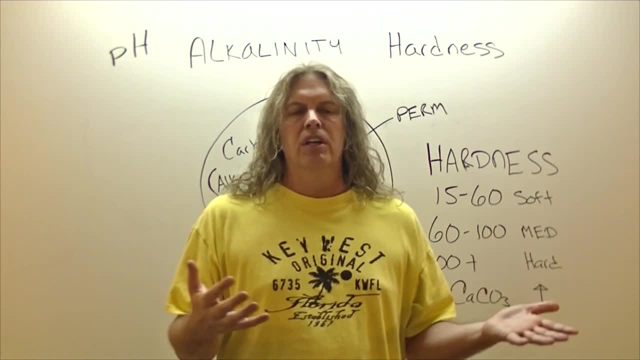 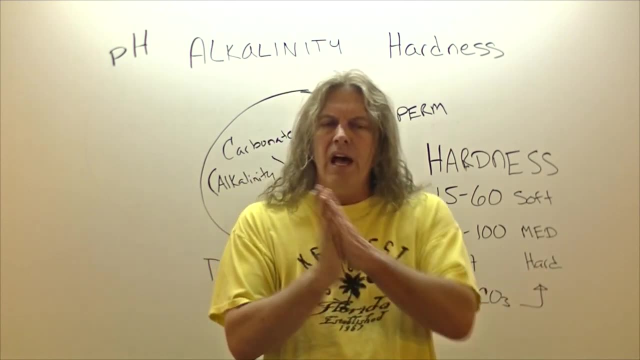 can't really see that. You can't really see that in the water. It's not a good thing, because calcium and magnesium in high levels are also the cause of hard water, which is very undesirable. Keeping an acceptable level is the trick We're. 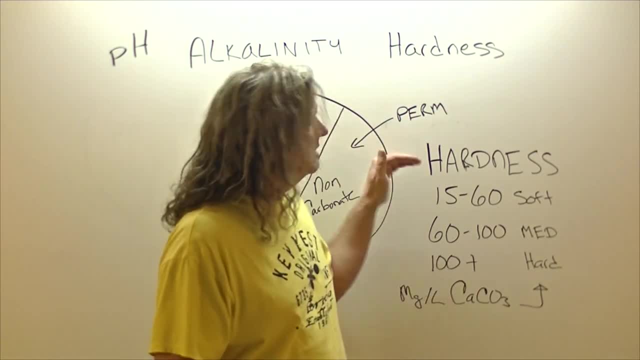 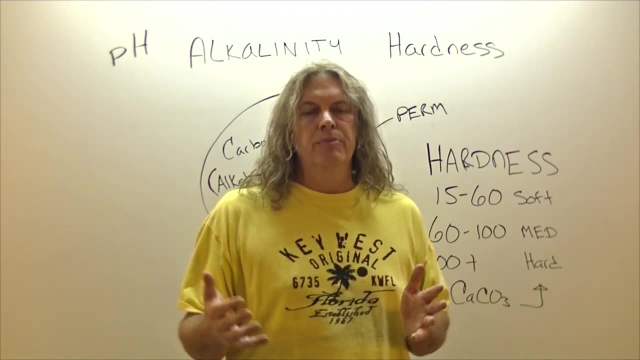 going to talk about how to do that in just a little bit, But for right now, let's talk about some guidelines on hardness and, like I said, these are just general guidelines. Again, calcium carbonate is measured in terms- excuse me- alkalinity is measured in terms of calcium carbonate. Hardness is also. 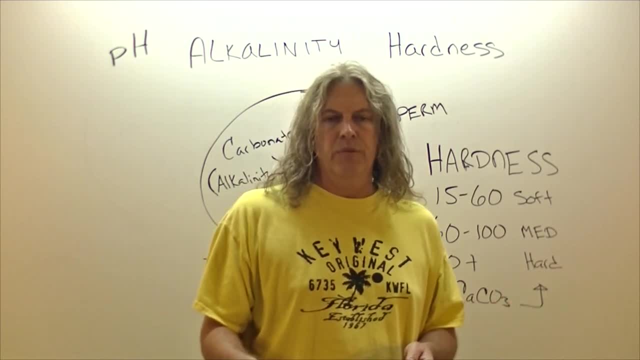 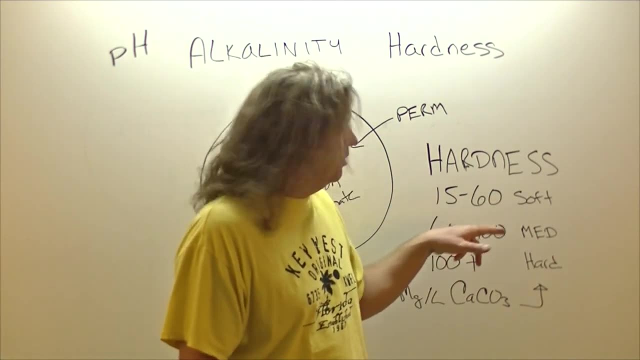 measured in terms of calcium carbonate or calcium carbonate. So it's just a little bit of a little bit of an example of calcium carbonate and it's expressed in milligrams per liter: 15 to 60 milligrams per liter of calcium carbonate or equivalent calcium. 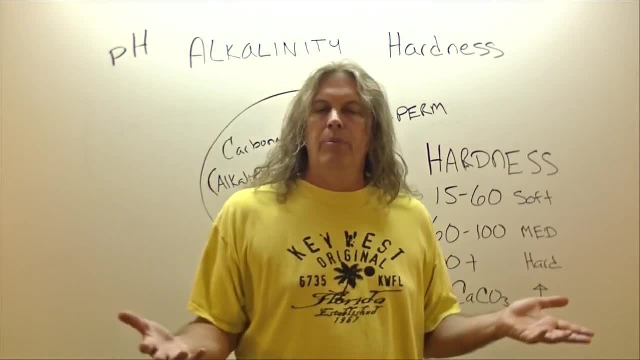 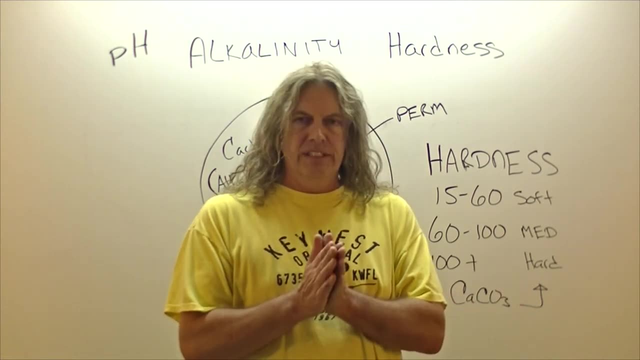 carbonate is said to be soft water. Now, soft water is very bad. It's very low in calcium carbonate, It's very low in alkalinity, It's very low in pH. It can also be very acidic and very corrosive, Like I said at the very beginning of. 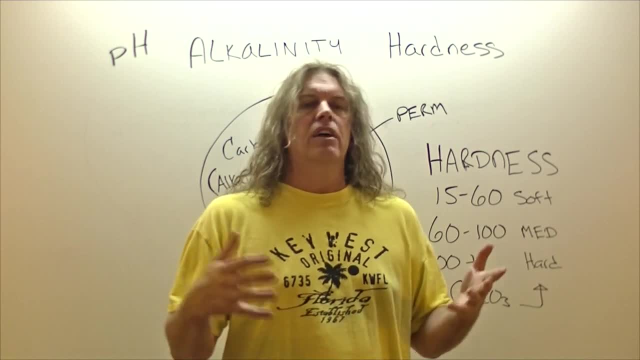 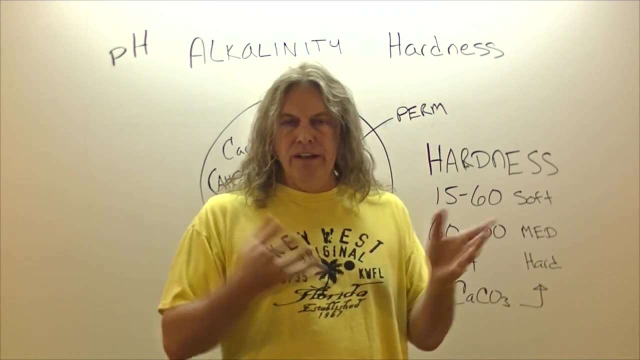 this video. acidic waters can eat away at the mains, It can cause holes, It can cause all kinds of damage from main leaks and so forth. But in addition to that they can leach the lead and copper out of pipes and into the water and you can consume a certain amount of. 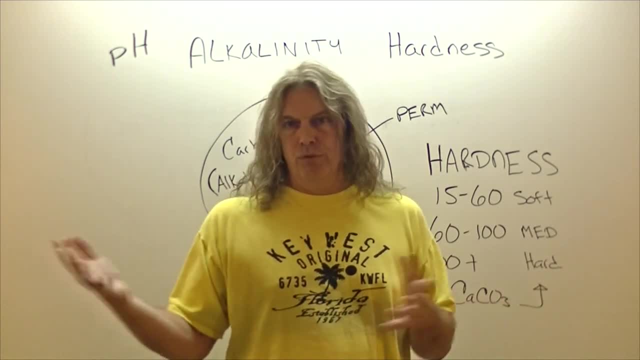 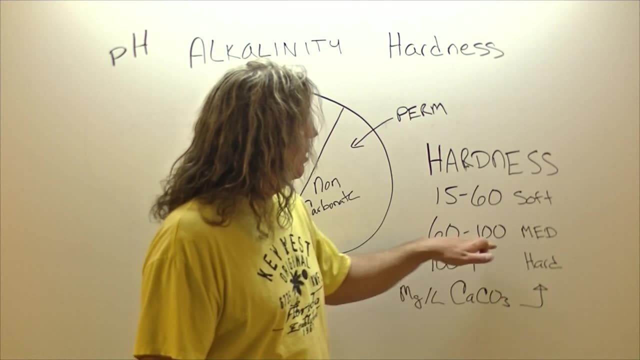 that when you drink the water, Lead and copper are bad for you. That's why they have rules and regulations regarding the maximum amount of that that can be in the water: 60 to 100 milligrams per liter of equivalent calcium carbonate. that's your. 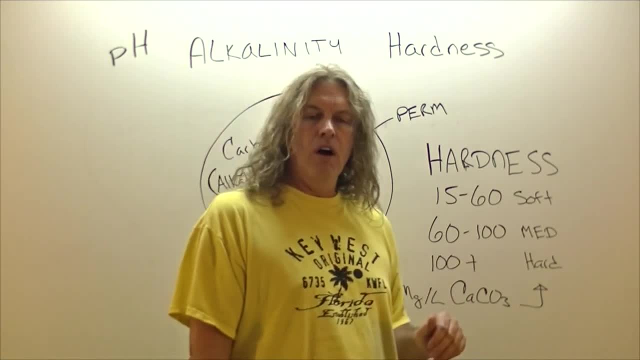 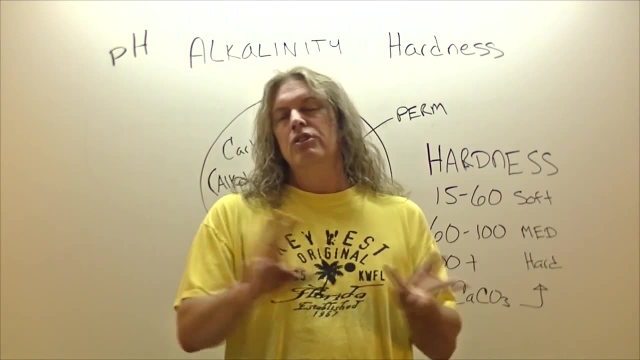 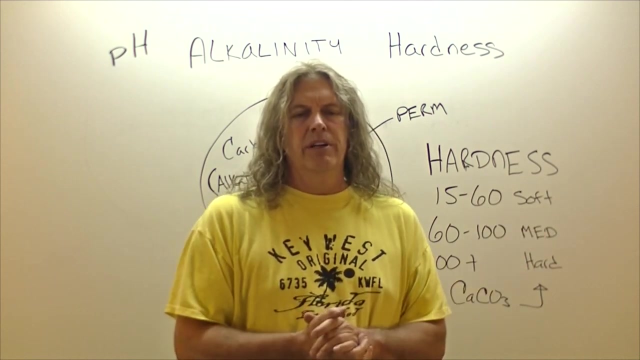 sweet spot right there. 100 plus is considered hard water, and hard water is not good It either. These are waters that are high in calcium carbonate, super high in alkalinity and high in pH. When your waters are high in pH and high in alkalinity and calcium carbonate, 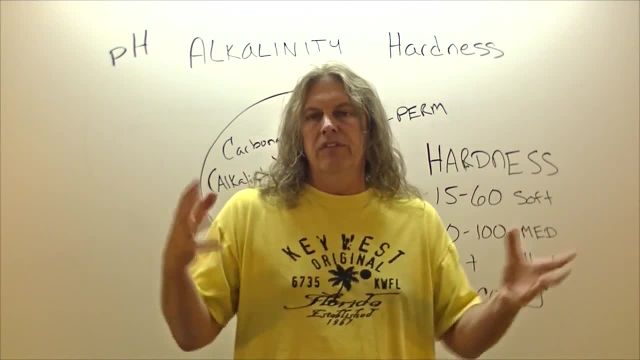 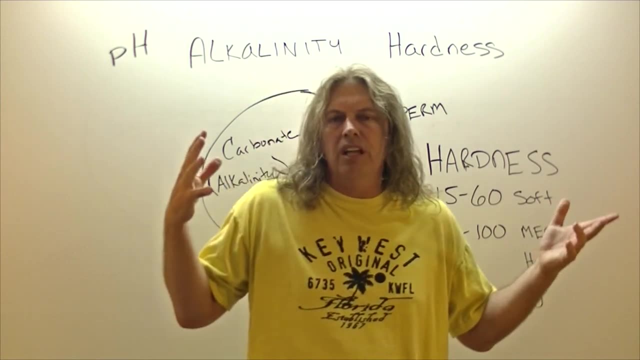 and all that. they can cause a formation of soap curds, actually stuff that comes out of the water. It can cause an increased use of soap, mainly an increased use of soap, because they stop soaps from lathering up. It basically stops that lathering process and inhibits the 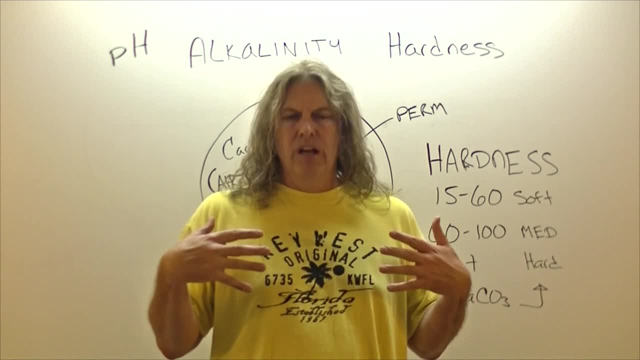 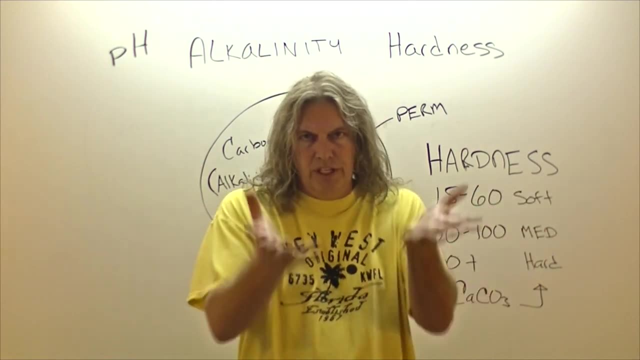 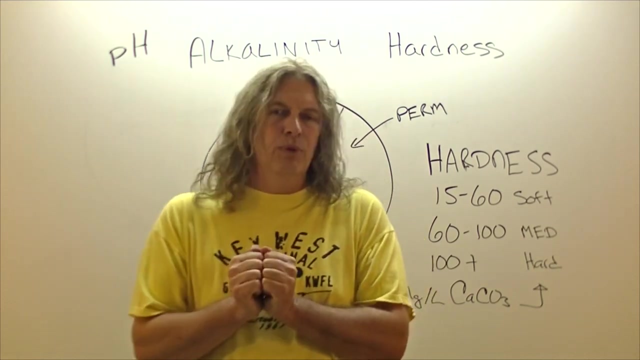 cleansing action. It also causes a deposition of the soaps. It also causes a deposition of scale in boilers, because when they heat it up they can just become saturated and come out of the water into an actual physical form. It causes clothes to lose softness or elasticity. This is where 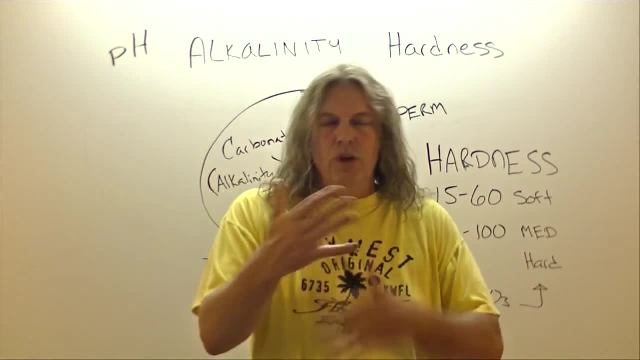 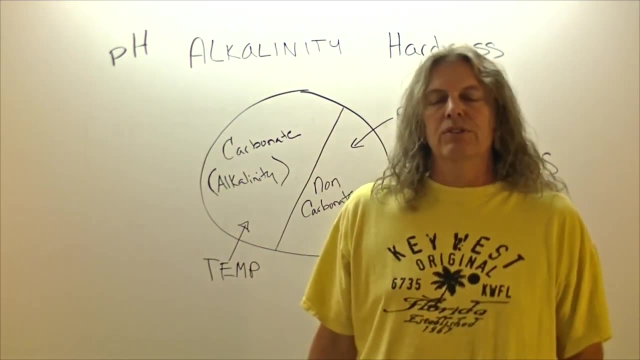 the actual homeowner, the average consumer. they notice that their soap is not sudsing up and that their clothes isn't soft. It's kind of stiff. They're walking around like Wally the Puppet Boy in their clothes and their underwear are rough on them and that. 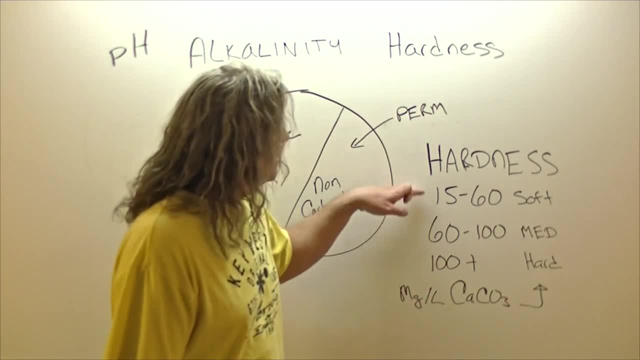 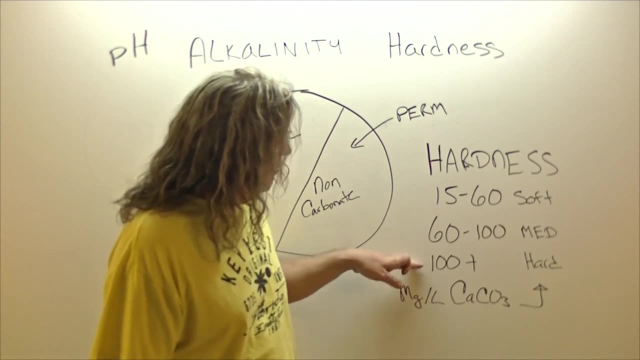 kind of stuff And people don't like that. So one thing about these guidelines: 50-60 saw, 60-100 milligrams per liter of equivalent calcium carbonate medium. 100 plus is hard. These are general guidelines And I see these. 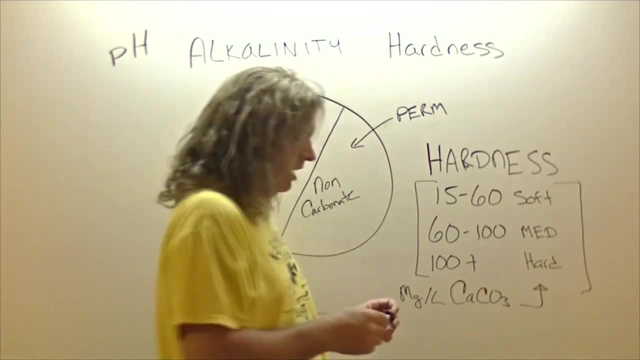 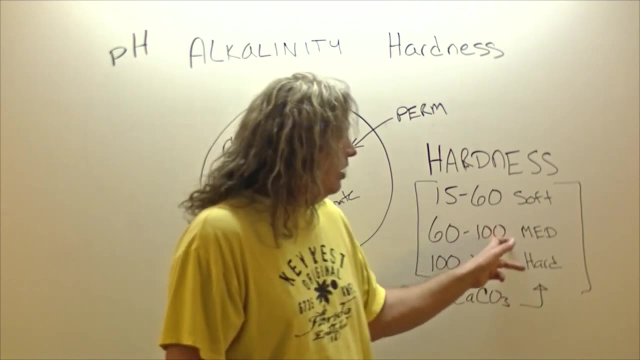 things all over the place, but that's just kind of a general rule. I've seen soft water considered something that was under 80 or 90.. I've seen medium go from 90 to 120.. I've seen hard be 120 to 120.. 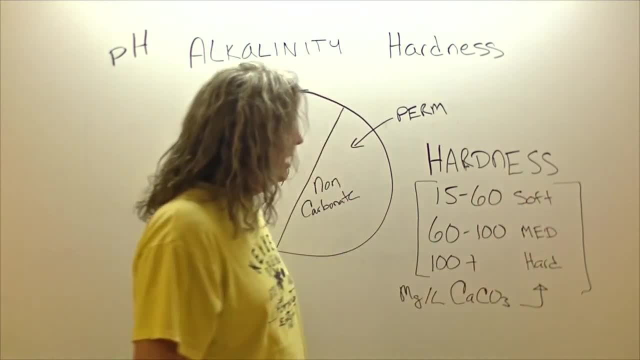 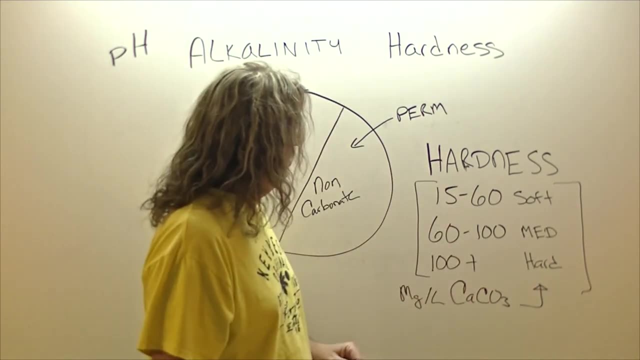 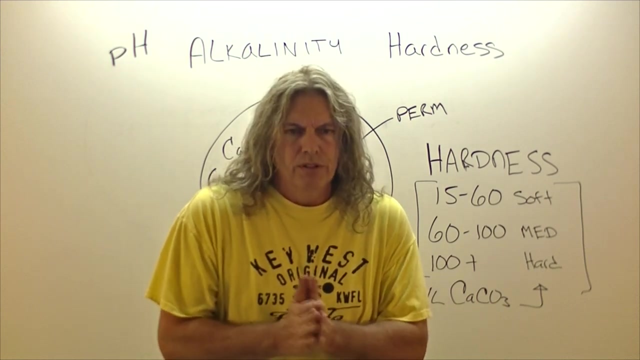 30 plus. so you'll see these kind of vary. just keep in mind- and that's the good ballpark- people generally aren't going to give you as a question like 60 and ask you to tell that one way or another. so let's talk about the forms of hardness. right now, hardness generally comes from calcium and 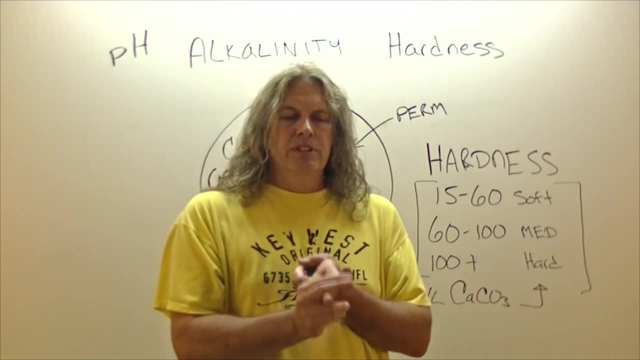 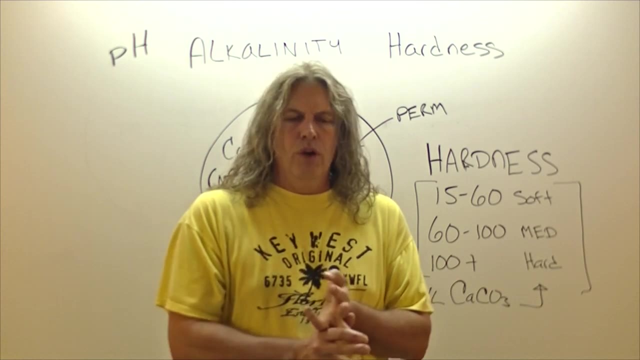 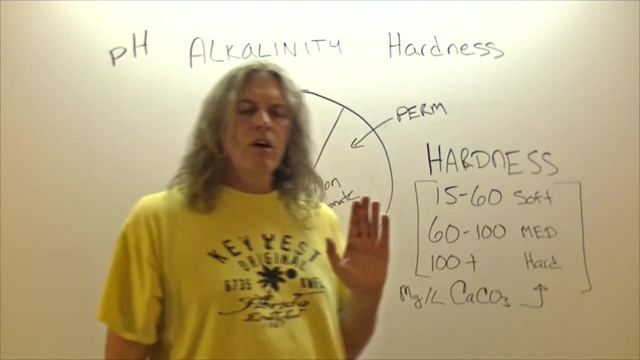 magnesium again, and there's three forms that it comes in: calcium carbonate hardness, non carbonate hardness and total hardness. and that's what this lovely little thingamajigger over here is for. just to kind of explain that now, carbonate hardness is caused when calcium step over. this way, carbonate 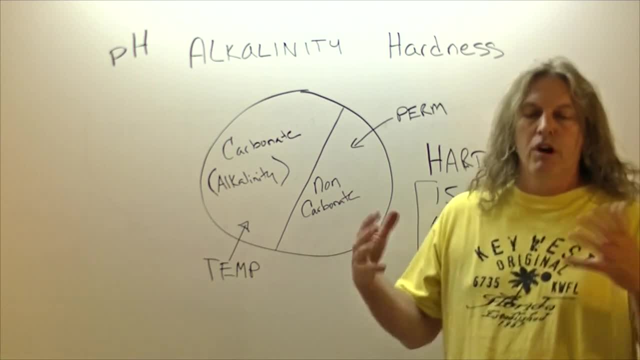 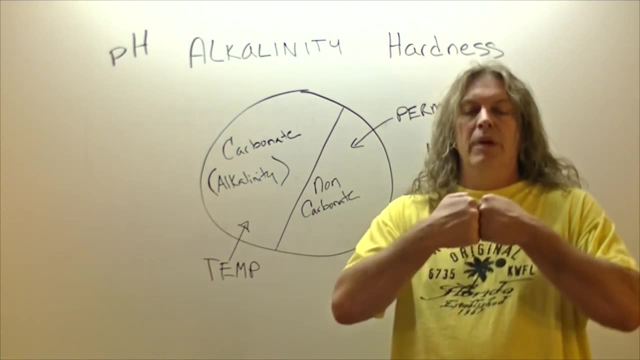 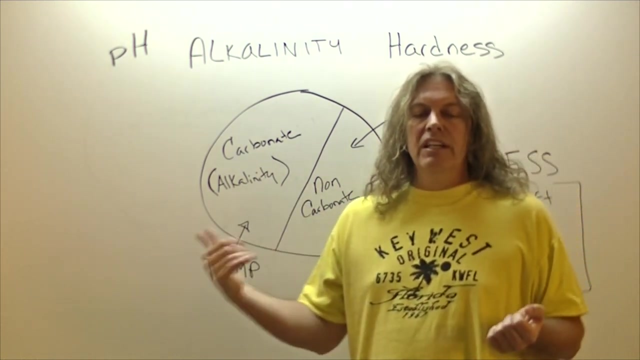 is. hardness is caused when calcium and magnesium bond with carbonate and bicarbonate ions. as I mentioned before, alkalinity results primarily from the bond of calcium magnesium with carbonates and bicarbonates, and it's also measured in terms of calcium carbonate, so alkalinity in the water. 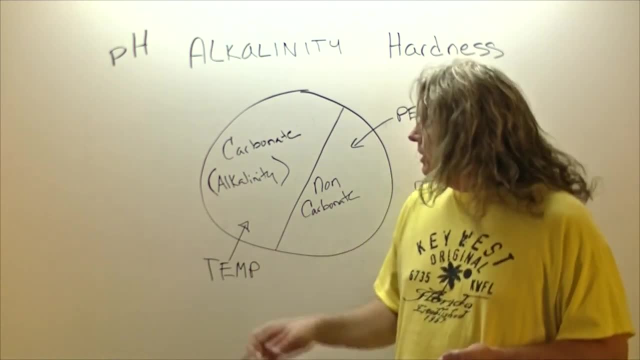 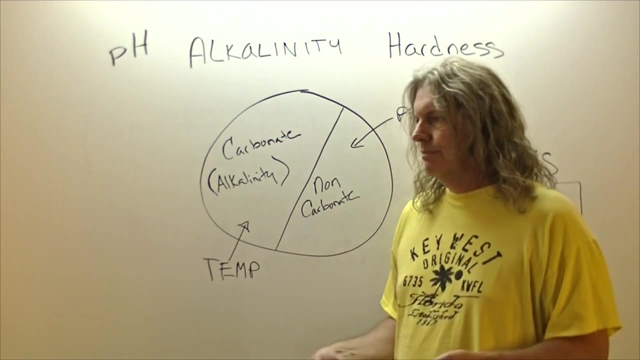 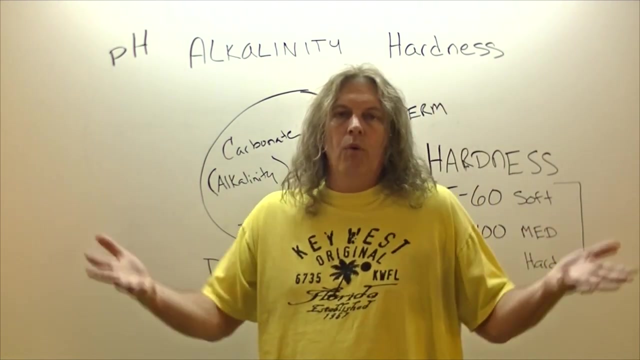 will equal the carbonate hardness. this is termed temporary hardness because, like I was saying before, it can be boiled out of the water into an actual. so what I'm thinking about here- I don't know what the word I'm thinking of, but it can be boiled out of the water in a 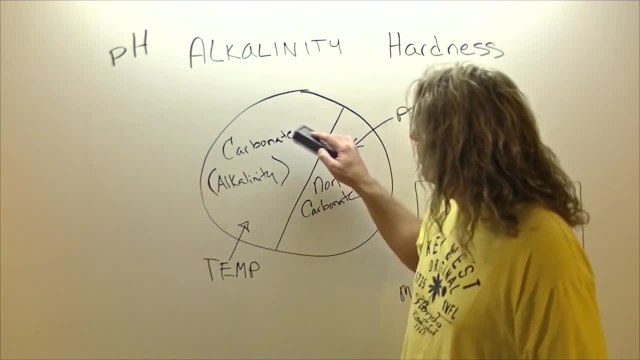 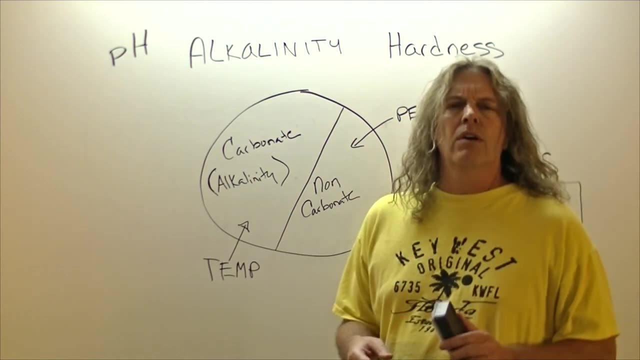 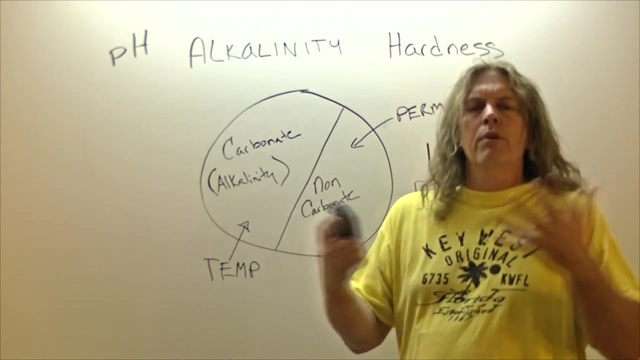 particulate matter. hey, that sounded good, okay, so carbonate water Is equal to your alkalinity. it's termed temporary hardness because it can be boiled out of the water now. non carbonate hardness represents the calcium magnesium that is bonded with other things other than carbonates and bicarbonates, so this is the calcium. 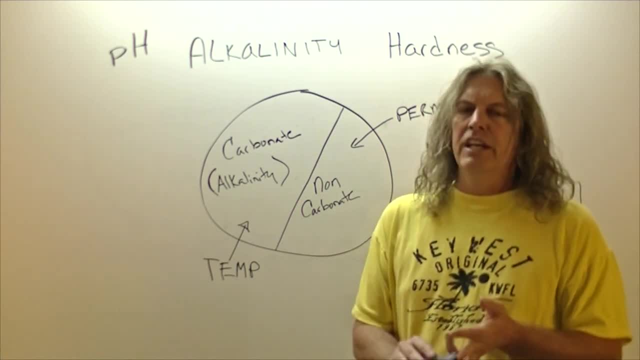 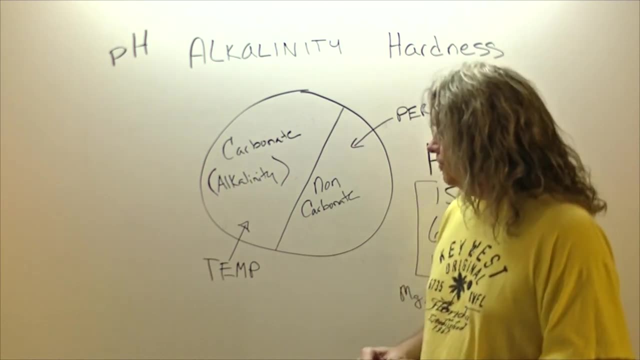 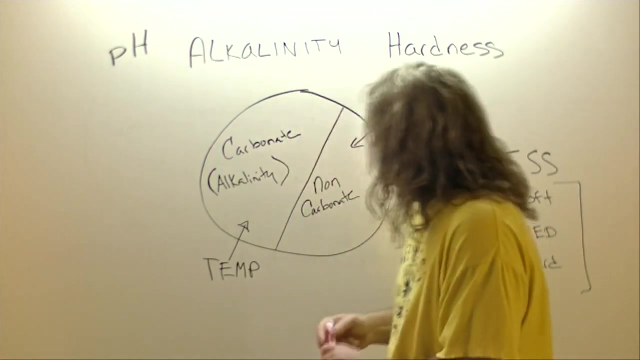 magnesium that is bonding with sulphides, chlorides, nitrites, things like that, and that is termed permanent hardness. because it can- permanent hardness cannot- be boiled out of the water. So if this is your carbonate hardness and this is your non-carbonate hardness, then the combination of all of that is termed. 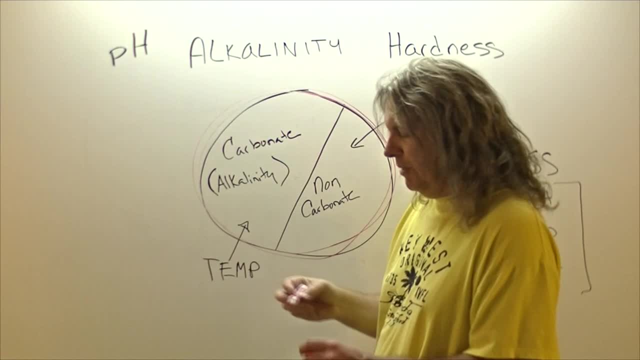 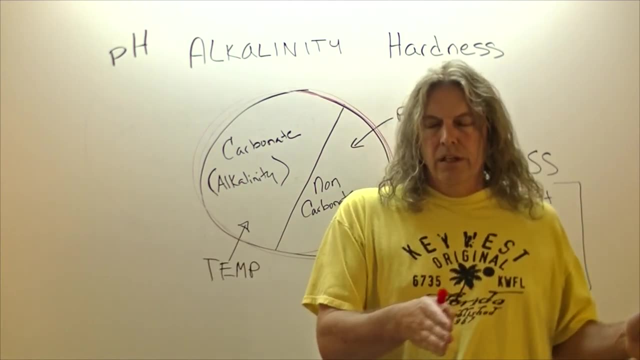 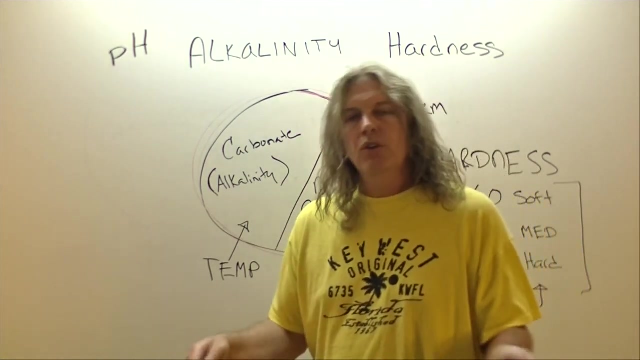 total hardness. So total hardness is your combination of your carbonate hardness plus your non-carbonate hardness. I kind of like to think of it as like the chlorine, You have your free chlorine, you have your combined chlorine and the two of those together add up to total chlorine. If you have no idea what I'm, 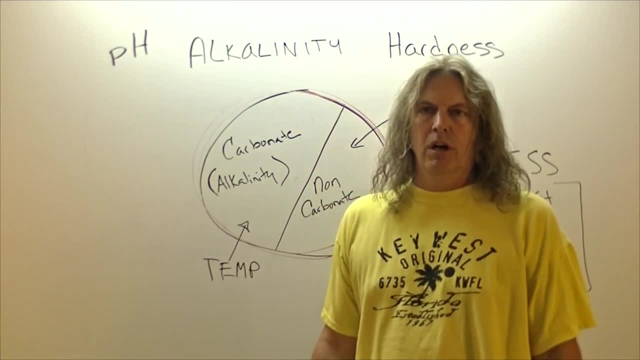 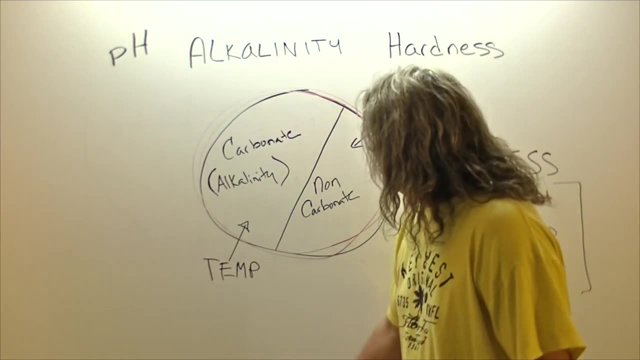 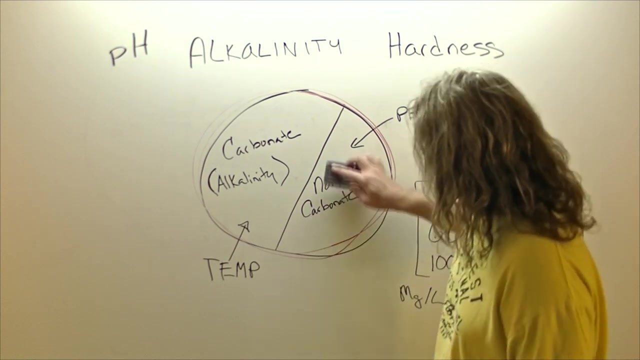 talking about. please, before you take a test, go watch my video on breakpoint chlorination. It'll save your life- Well, not literally, but it'll save your test. Okay, now just another thing to think about that with relationship to that. If there is no non-carbonate hardness, this is kind of simple, if all. 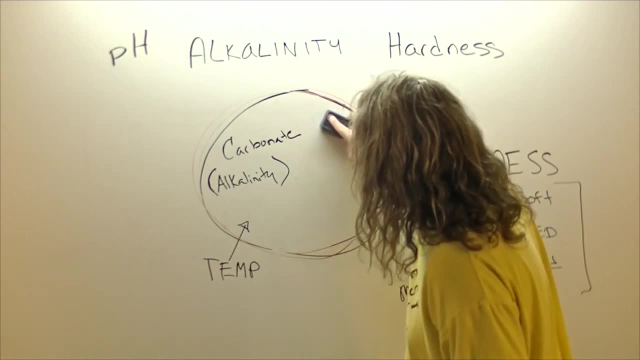 the hardness in the water is in calcium carbonate form, then you have a non-carbonate hardness. If there is no non-carbonate hardness, then you have a non-carbonate hardness. If all the hardness in the water is in calcium carbonate form, 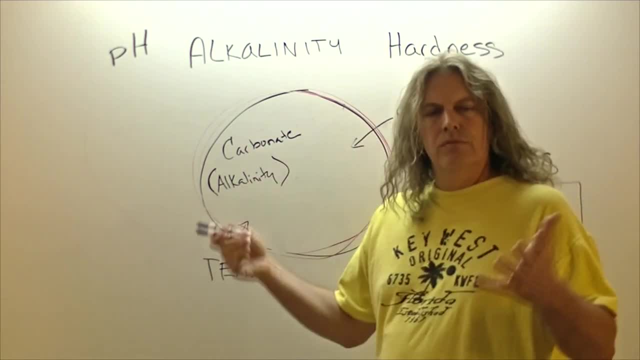 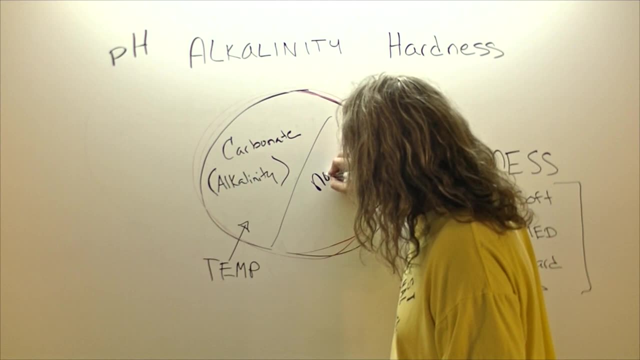 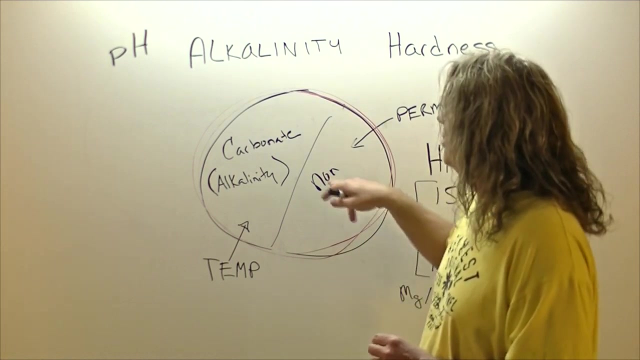 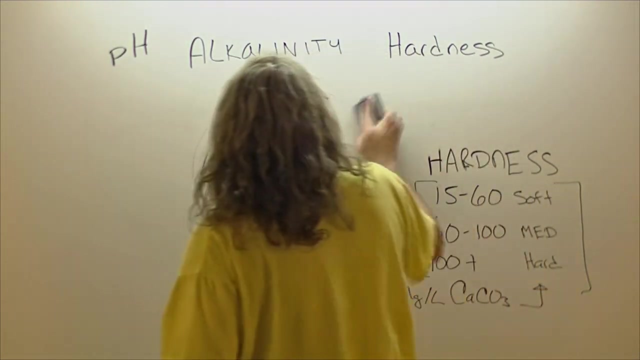 then carbonate hardness equals total hardness. If you have more, then obviously your carbonate hardness plus your non-carbonate hardness would equal your total hardness. Let's talk a little bit about carbonate saturation in water and how we actually measure that. I think I might mess up. 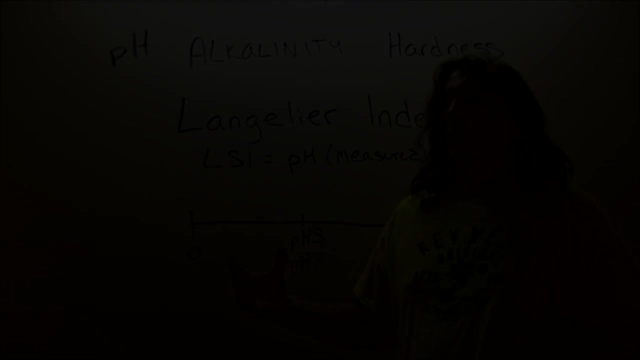 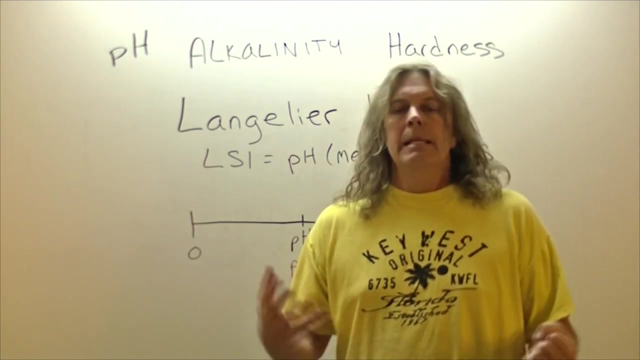 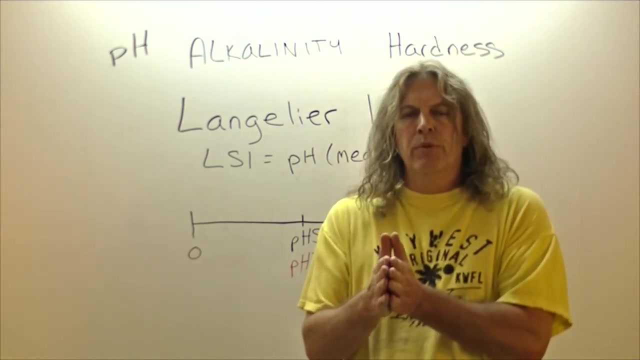 I created a new mess. So, wrapping things up, I want to talk about that calcium carbonate saturation in the water and how we exactly measure what that is so we know what to do with it. We talked earlier about the balancing act of calcium carbonate with regards to hard and soft water, and we talked about how. water is considered stable when it's a perfect saturation of calcium carbonate at a given pH. Now, perfect equilibrium in the water is neither scale forming or is it corrosive. If pH is raised from that point and everything else stays equal, the carbonate participates. 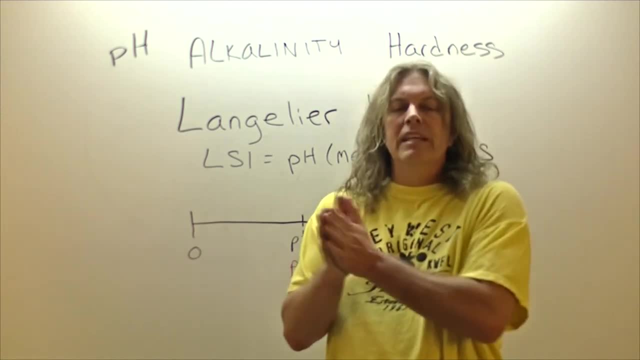 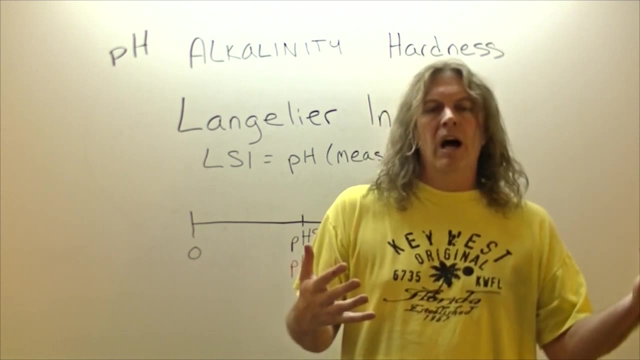 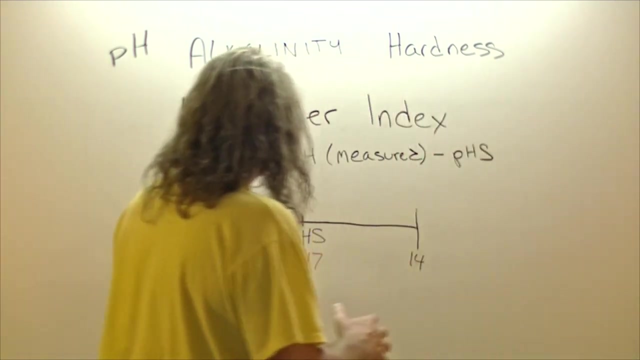 the carbonate precipitates out of the water and it actually becomes scale forming. This causes a layer scale to deposit on the inside of pipes and boiler process stuff like that. If pH is lowered, the water becomes corrosive. Now remember when we talked about pH. 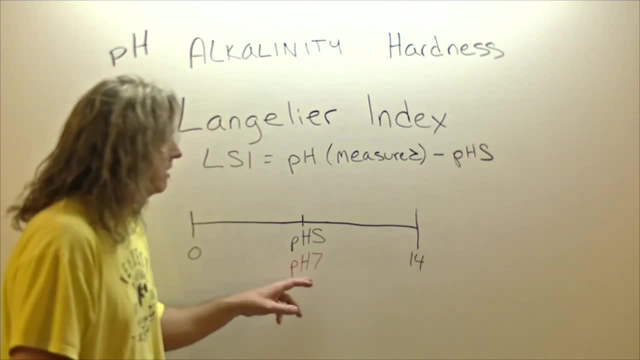 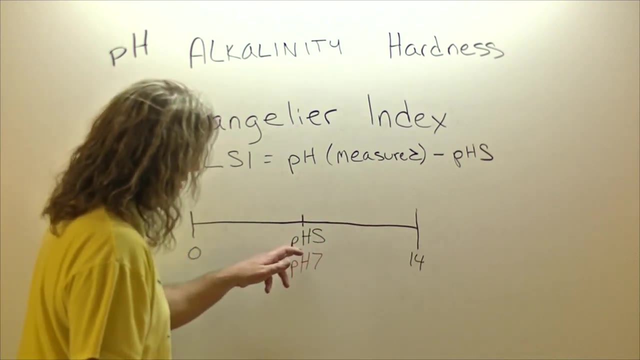 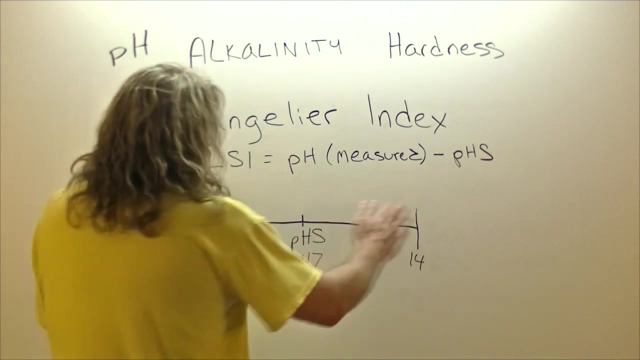 at the very beginning and we said a water of pH of 7 was neutral waters. It's neither acidic nor is it basic. Let's assume for a second that the pH of saturation would be equal to the pH of 7. Then it would be the exact same thing and it's really simple. So if the pH at saturation was 7,, then anything greater than that would be scale forming or basic would make it more scale forming. Anything less than that would make it more acidic. So that it should be kind of a simple way to go: Your pH and saturation basically just adjusts this neutral point around and everything else. 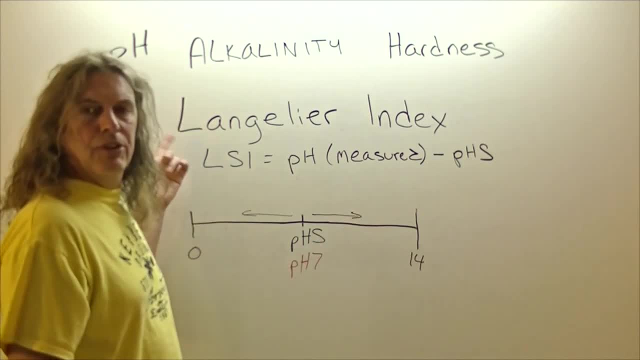 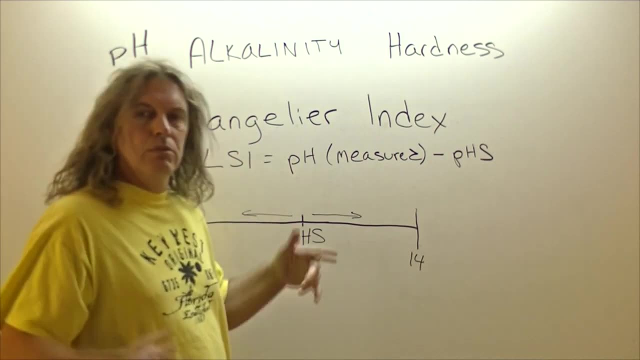 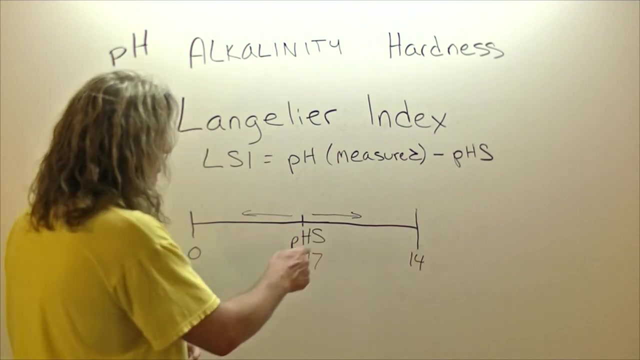 kind of stays the same way. So in like 1936 along comes this guy, Wilfred or William Langdon Langolier, and finds a way to make this really confusing. Then he names it after himself and now we got to learn it all. But really all it does is move that equilibrium point around. 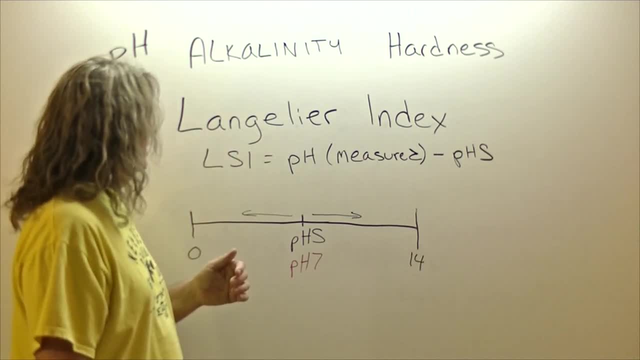 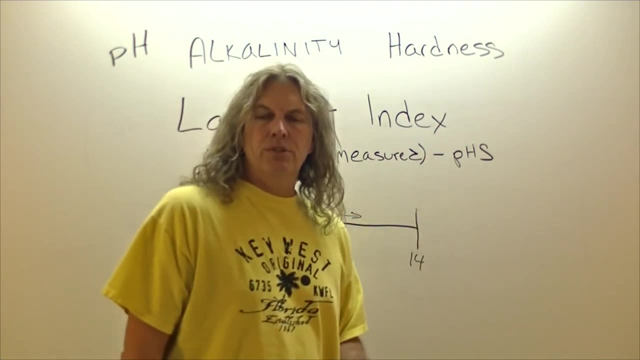 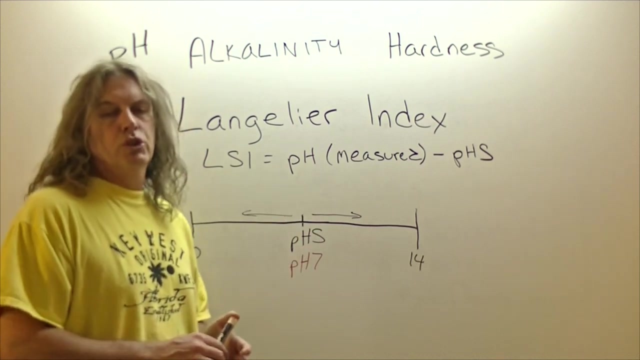 and basically he invented this Langolier index. Langolier saturation index equals the pH measured minus that pH at saturation. Let's talk about how this works real quick. For example, let's say your pH, that you actually measured into the pH at saturation. So you're measuring the pH at 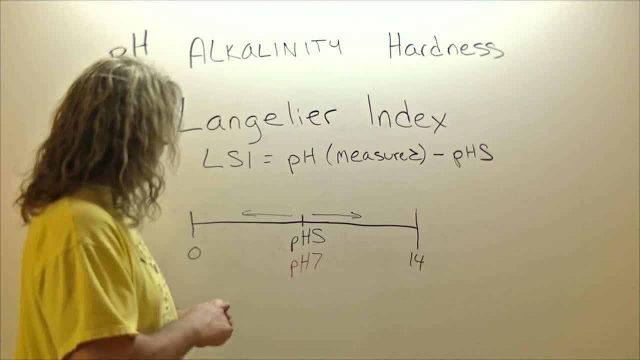 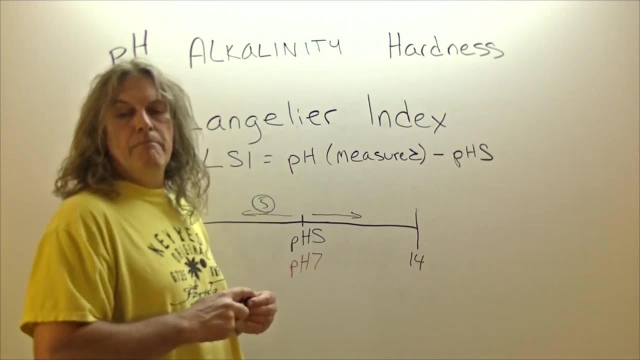 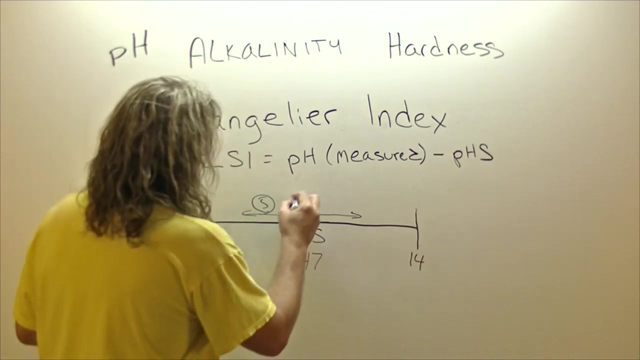 5. That pH in the water was a 5.. So you went out, you took your water sample and your measured pH is a 5.. But that perfect saturation point is a 7, just like we had right here. So the perfect saturation is 7.. 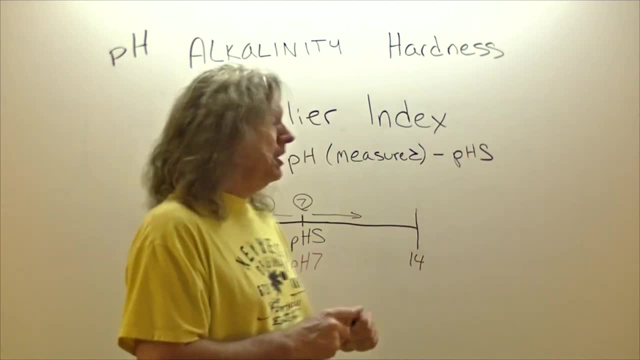 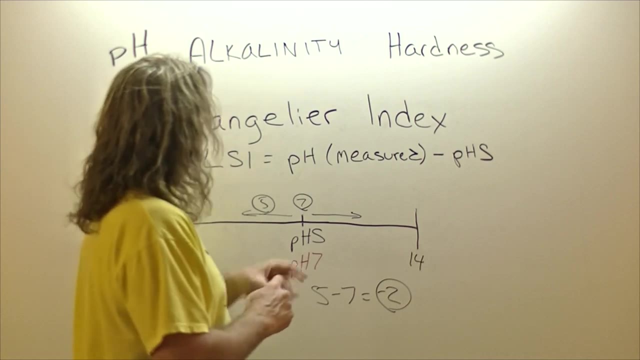 Then what we would have is our measured pH minus our pH at saturation, 5 minus 7. And that would equal a negative 2.. Now, according to the Langelier index, a negative number means that the water can be corrosive. 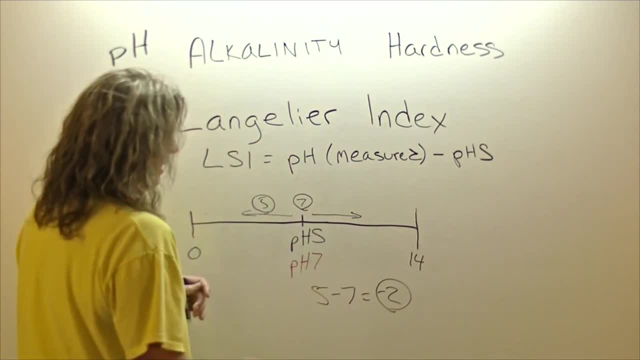 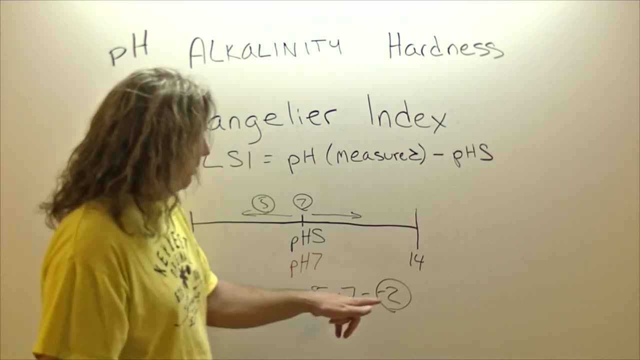 no different than we could have figured out here just by going like we did. If the pH was 7 and we were less than the neutral point, it's negative and it's corrosive. So you'd need to increase that pH by 2 to bring it back in equilibrium. 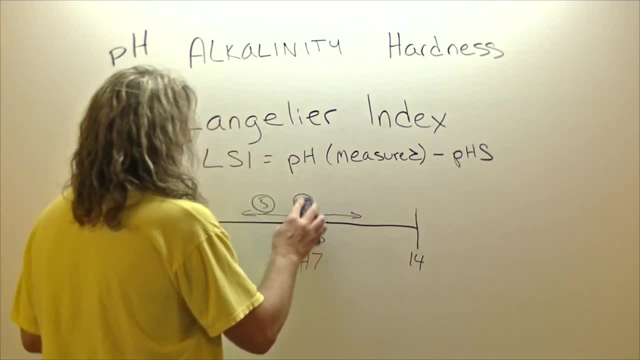 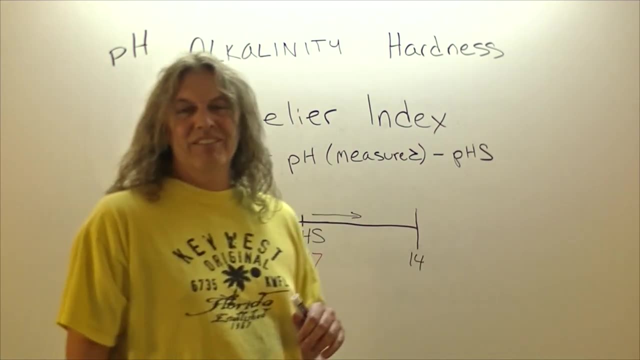 Just on the opposite side of that, let's do another one, because Mr Langelier made this so fun. I'm sorry, I don't mean to go off on him so much, It's just some things just seem needlessly confusing. 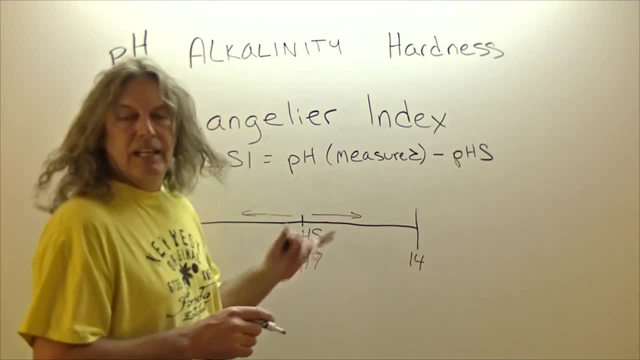 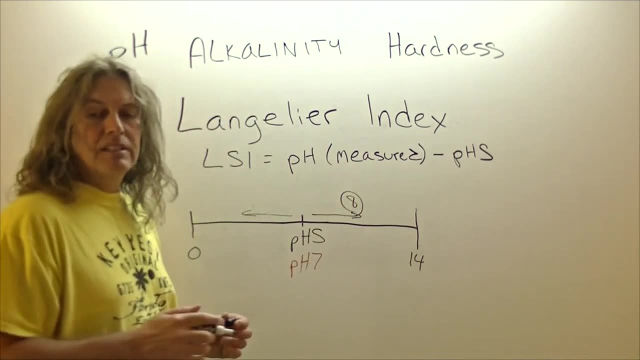 So let's say the pH measured is at 8 this time. So let's say our pH that we measured in the water is up here at 8.. And this time, instead of our pH at perfect saturation being like the ideal world, was at 7,. 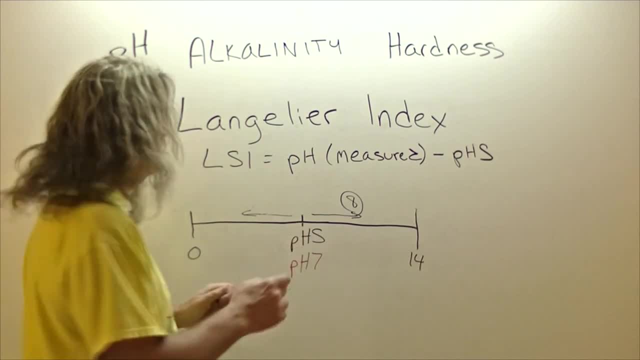 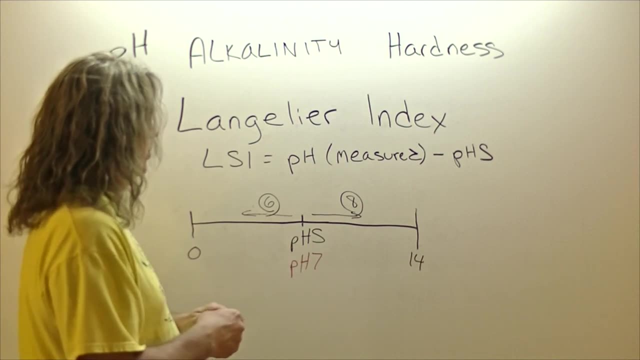 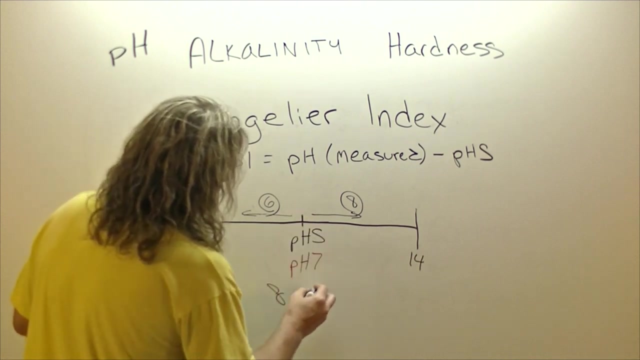 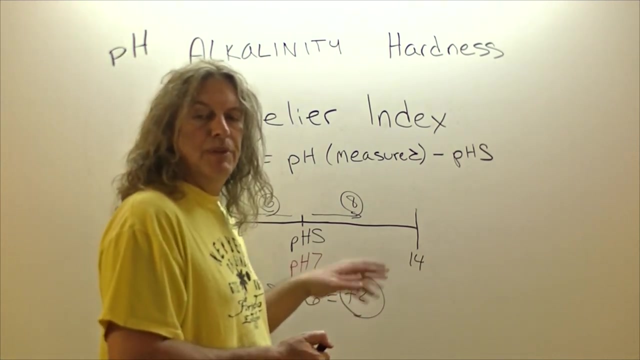 this time our pH at perfect saturation is 6.. So now what we have is the pH measured, which is 8,, minus the pH of saturation, which is 6,, and you end up with a positive 2.. Now, under the Langelier index, positive numbers means the water has a tendency to form scale. 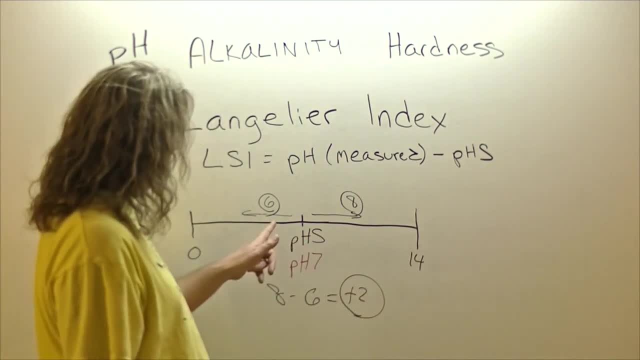 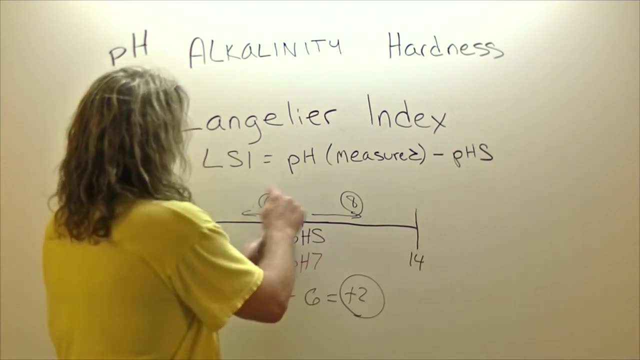 Rather than doing all this, it seems so much easier just to move that saturation point over and look at it there. So if this is if the perfect saturation or the equilibrium, if the equilibrium point is 6, and we're 2 above that, that's a 2.. 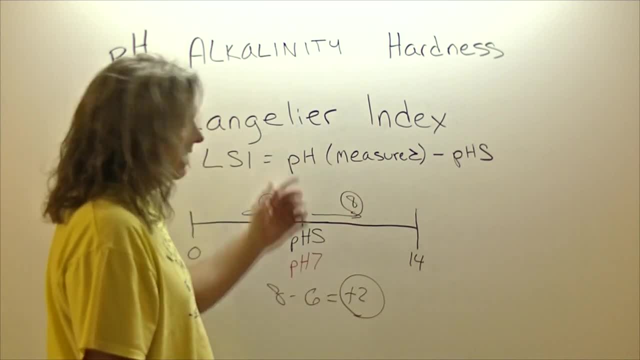 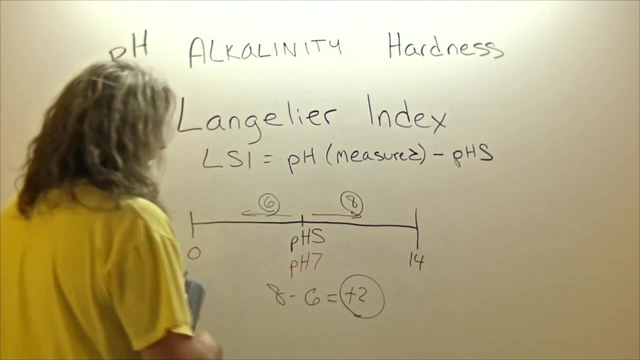 And not only that, but if you're on this side, then it's scale forming. That's kind of another way to think about it. So that's the Langelier Saturation Index. The last thing I want to talk about is the Marble Test. 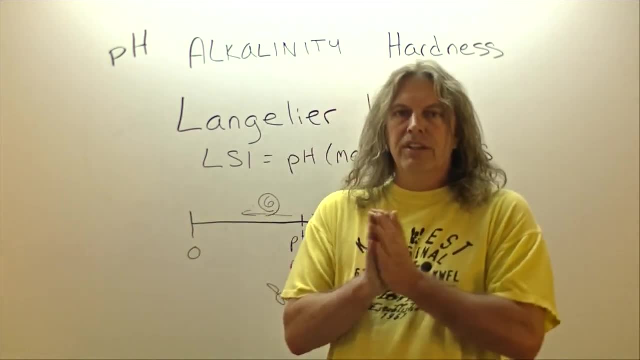 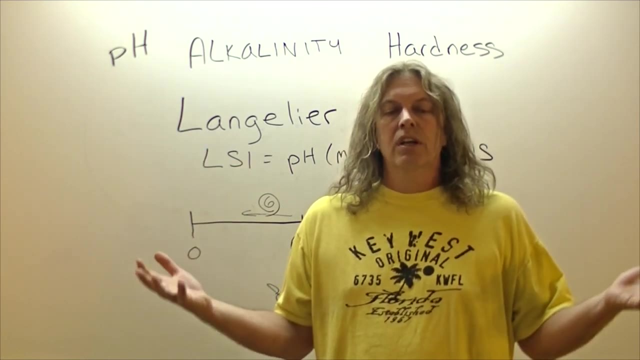 And the Marble Test is one of the simpler methods of determining calcium carbonate saturation. It directly measures whether water is going to increase in hardness and pH when it's dosed with calcium carbonate. So very simple, A very, very simple five-step process. 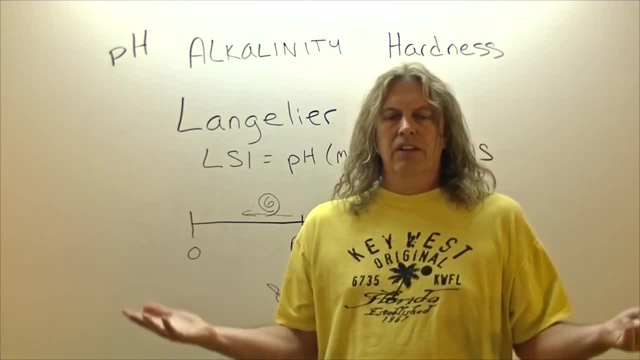 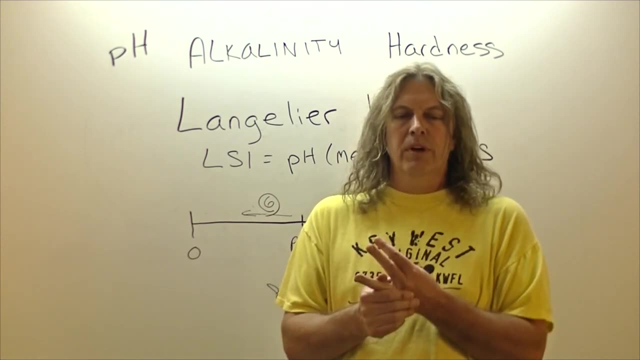 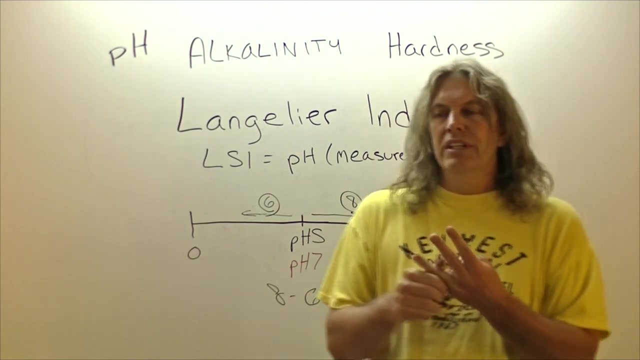 One, you measure the pH, the alkalinity and the hardness of the water. Two, you add calcium carbonate and then you stir the water. And three, you re-measure the water for pH, alkalinity and hardness. If they've increased, that means that that calcium carbonate that you added was absorbed into the water. 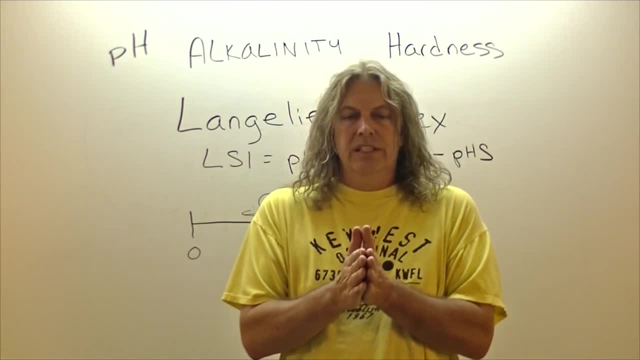 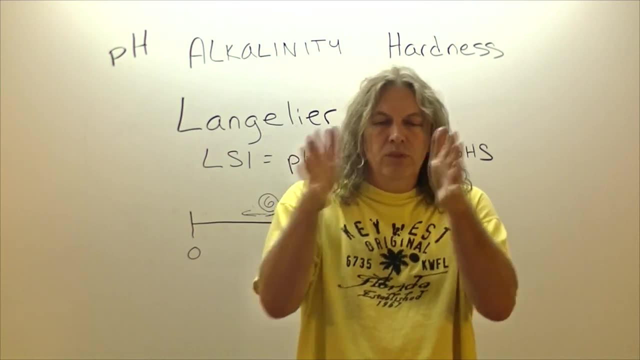 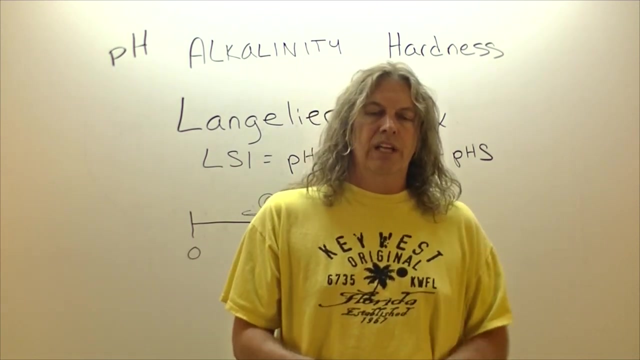 It was under-saturated. If they decrease, it was super-saturated. Now, by decrease, what I mean is your initial dose plus what you added was kind of down. Some of that particulated precipitated out, And so you know it was super-saturated.